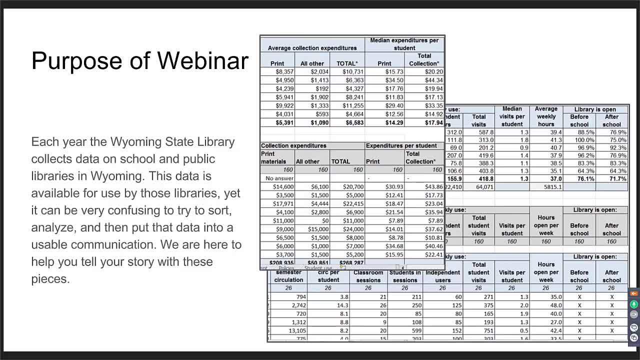 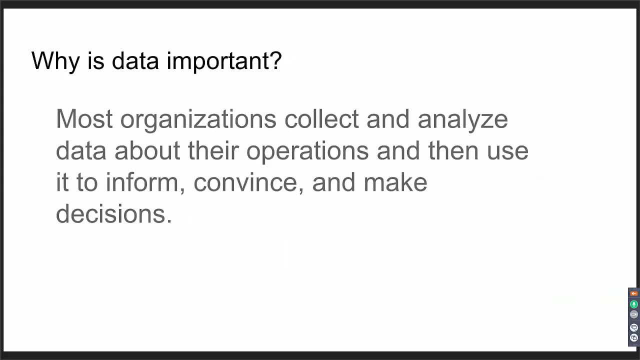 to sort, to analyze and to figure out what type of format to put it into. So we're here to help you use this data to tell your story. So why is data important? Most organizations collect and then analyze the data about their operations and they use that in order to inform, convince and 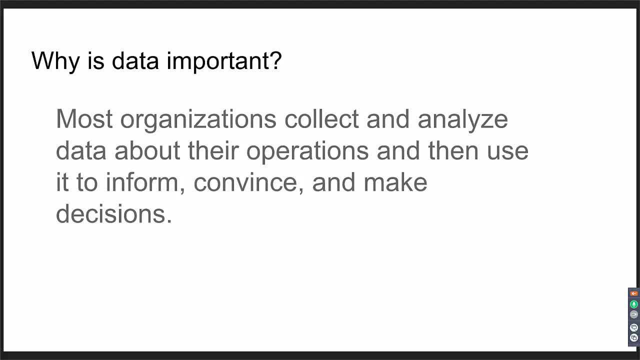 make decisions. But even if your organization doesn't collect data, you can use other sources that have collected. For instance, you could use data that has been collected by the Wyoming State Library, other state libraries, the IMLS and the state's National Book of Science experience. This is a request for any additional information. please send us any data you may have, without Area Decease, Just for furthercompliance. 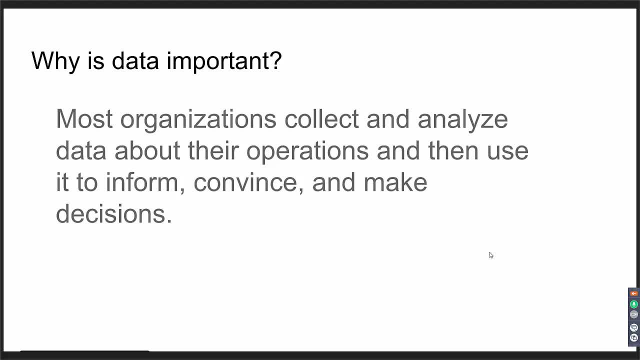 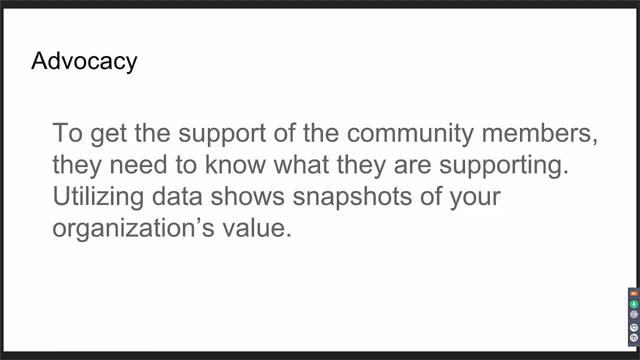 Wyoming Department of Education or whatever state you're in those sources, or the US Department of Education, and that's just to name a few. So we can use this data for advocacy purposes. When you wanna get the support of community members, they need to know what it is that they're. 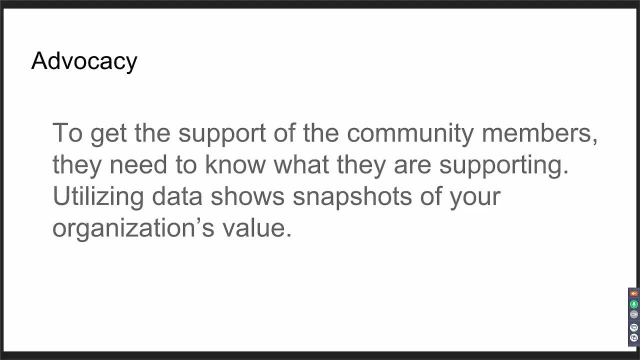 supporting. Using this data that is gathered will help show snapshots of your organization's value. Teton County Library shares with us that they have used data from community surveys in order to give them some guidance on developing their strategic plan, So you need to make your case when you're using data. 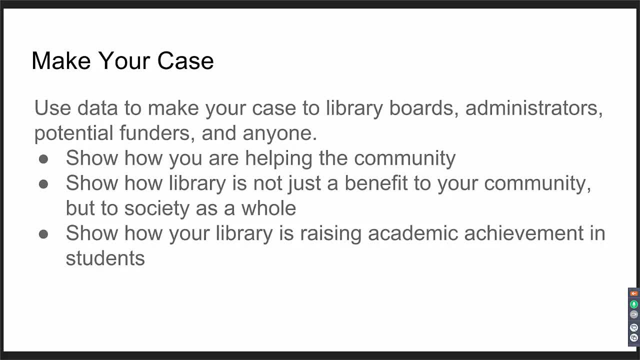 whether it's to library boards, administrators, potential funders or the community at large. Maybe you need to show why you need to increase a collection, So you need to pick your audience and then transform your data to that audience. The South Dakota State Library shared. 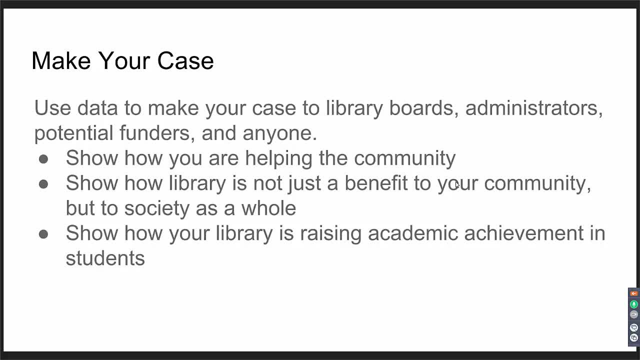 with us that more and more of their public librarians use public library survey data to support requests for staffing. They also get requests for larger material budgets and larger library spaces. Several of their librarians also contact the state library for help in using library statistics and comparison data when they 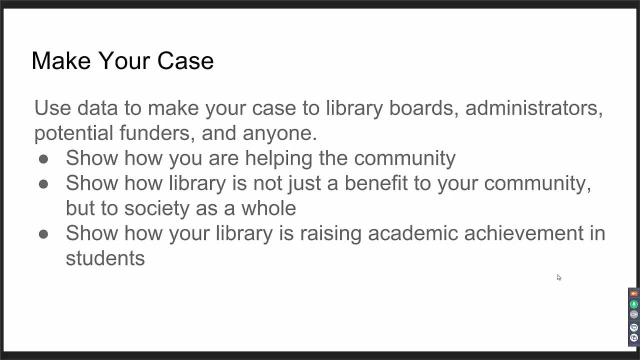 are presenting their annual reports to decision makers like the city or county commissioners or boards. They also shared with us that most of their requests for data from their school library survey is used for making comparisons. In fact, most state libraries, including Wyoming, produce some kind of summary for their individual. 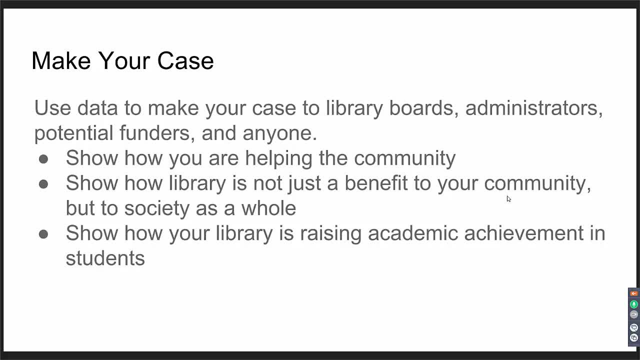 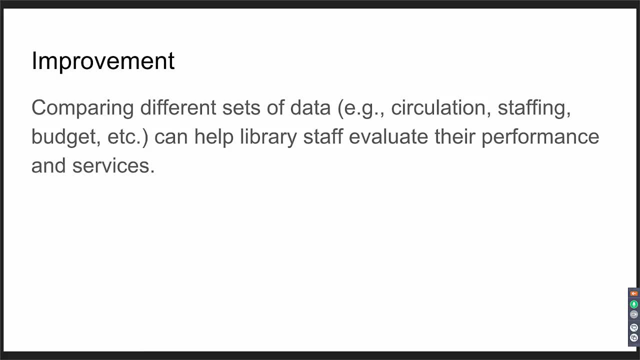 surveys. These summaries can be a good source of data. Data can also be used for improvement When you compare different sets of data, for instance circulation data or budget data. this can help your library staff evaluate their performance and services. A school librarian in Wyoming used data from the school library survey to help 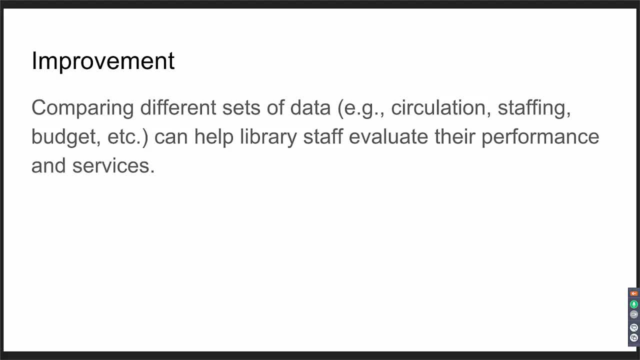 prevent a cut to her library budget. She printed out a spreadsheet with data from all of the participating schools, then highlighted the schools that were most similarly sized to hers. The data revealed that the age of her collection was older than those of the other schools. A drop in her budget would not. 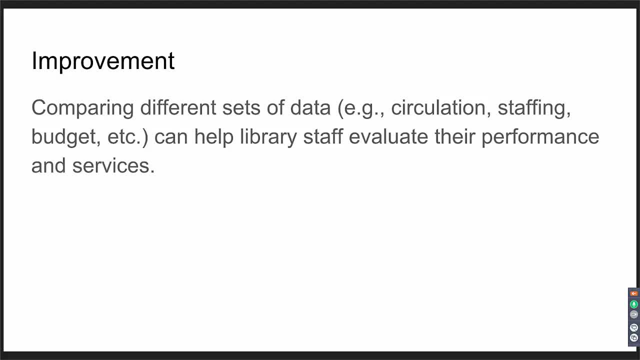 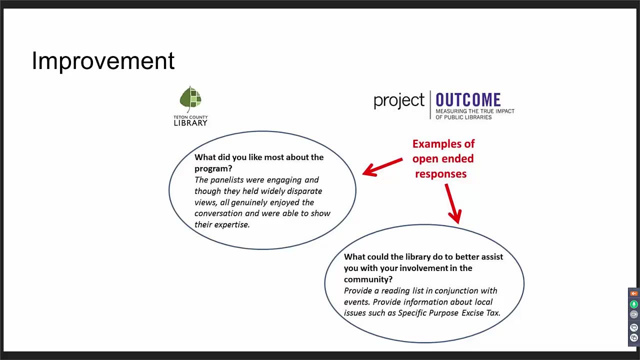 only put her below what their budgets were, but she already had some catching up to do in terms of updating her collection. It was effective in convincing her principal to not cut her budget that year. Some surveys include open-ended questions as well. You can get more specific. 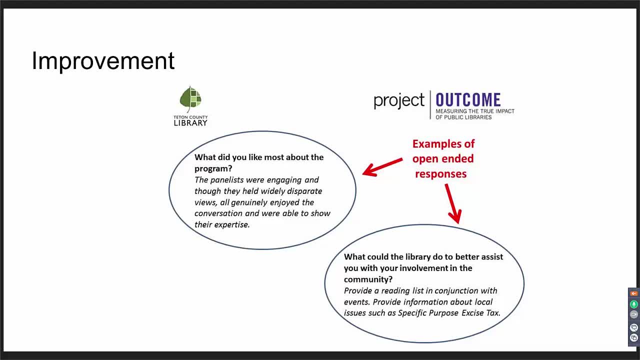 information by using open-ended questions. Here is an example of a couple of open-ended questions used by Wyoming's Teton County Library. They use project outcome to survey for their programs that they had done And one of the questions was: what did you like most about the program? And they can use 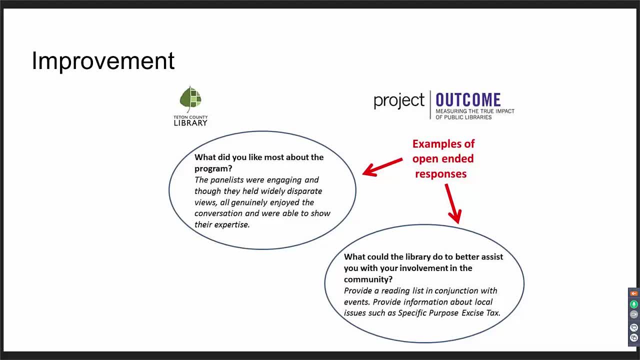 those to get specific information to aid them in making their programs better or maybe in choosing topics. They also asked: what could the library do to better assist you with your involvement in the community? These are examples of them putting out questions that aren't yes or no. they don't give you numbers, but they get. 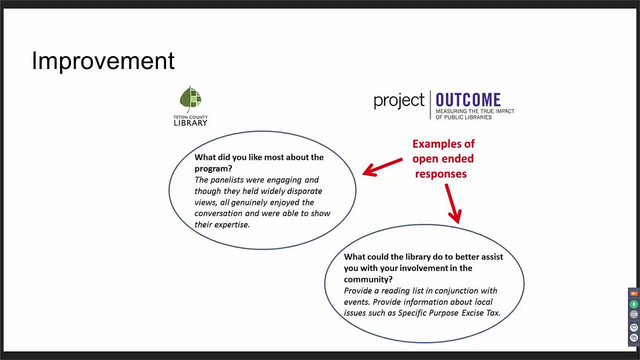 them more specific information that they can use, And certainly this type of information could be used when doing reports or, depending on the audience that you are reporting to, you would choose how you would portray it to them. So this is a reminder that not all data is numerical. 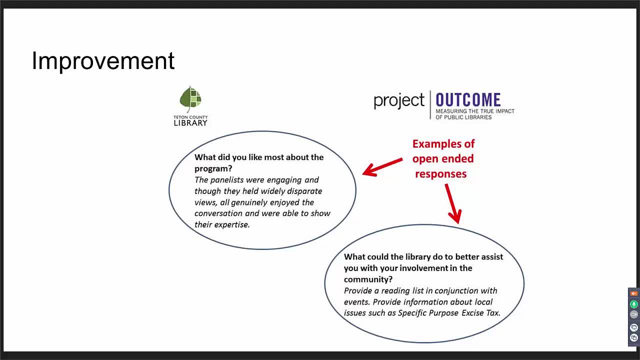 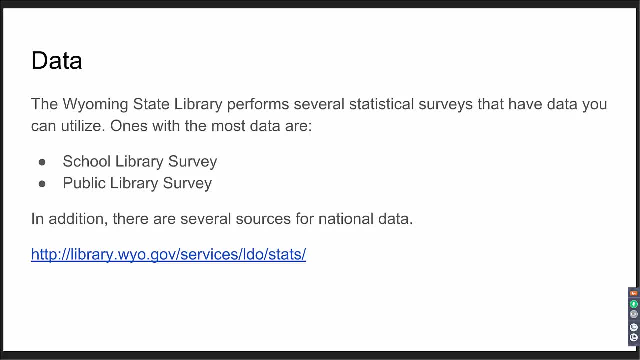 it can be text. There are lots of places to find data. Our most popular data sets at the Wyoming State Library are the School Library Survey and the Public Library Survey. These are great for Wyoming data, but maybe you want to use regional or national data. 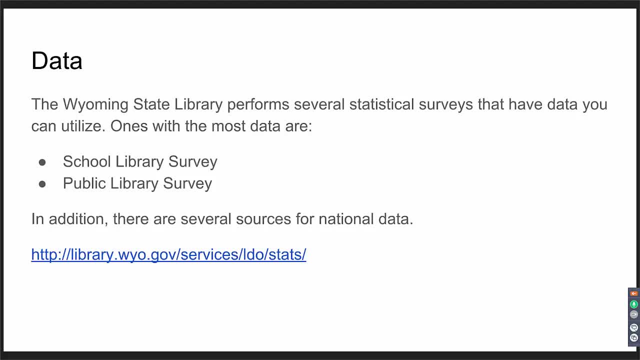 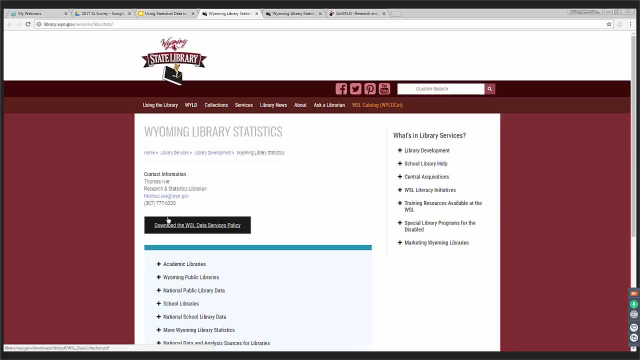 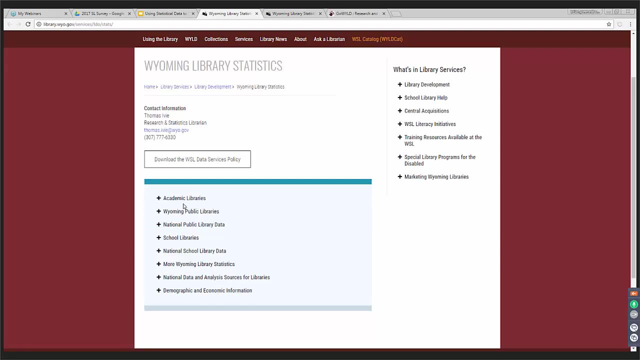 And we have links to several data sets on our website. So we'll just go to the Wyoming State Library's statistics page and go through a couple of our A few of our products. Like we said, we do have information on academic libraries. The NCES hasn't. 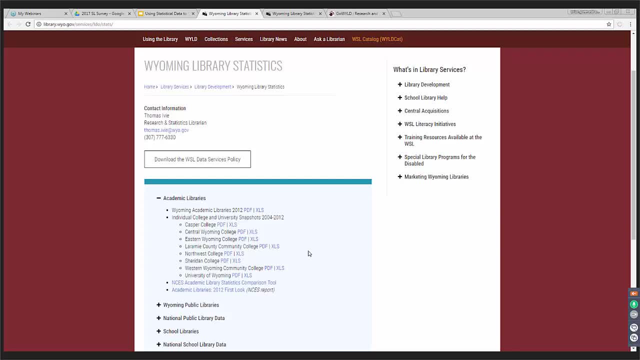 done a full survey since 2012,. but if you go to their website, they do have some smaller chunks of information on there that you could use. The Wyoming Public Libraries. we're in the process of getting the 2016 data in, but I'll go through the. We have the. 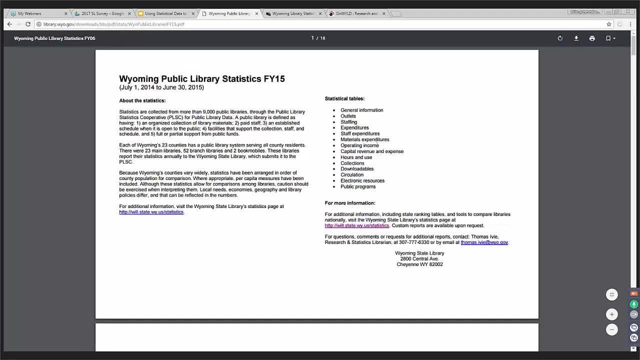 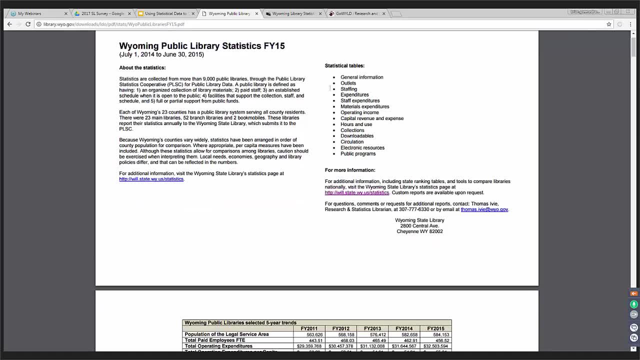 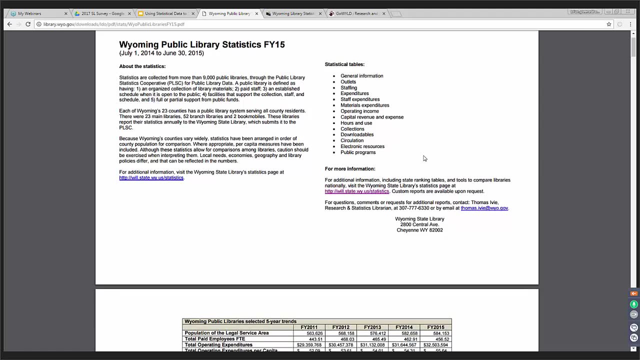 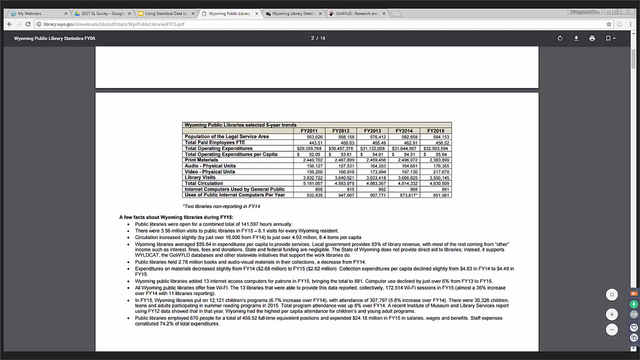 raw data And by looking at that. here's an example of a summary of the different tables, the different parts of information that we have in the survey. We give a five-year trend summary and then some facts about Wyoming libraries during that fiscal. 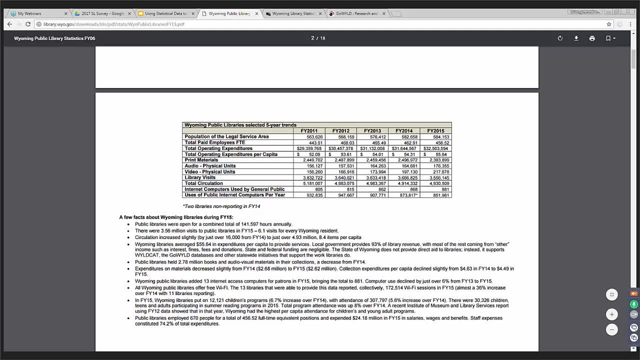 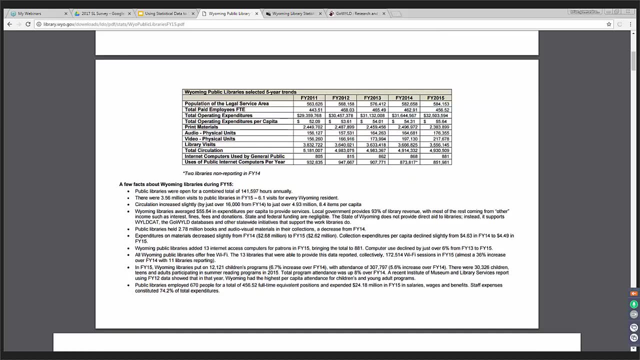 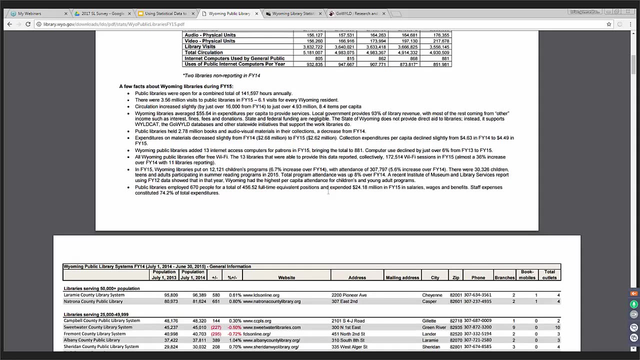 year So you can draw numbers from there. use that data. It's a quick way to get data and most states provide some kind of summary to their their data, because if you look at the raw data it can be difficult to understand. 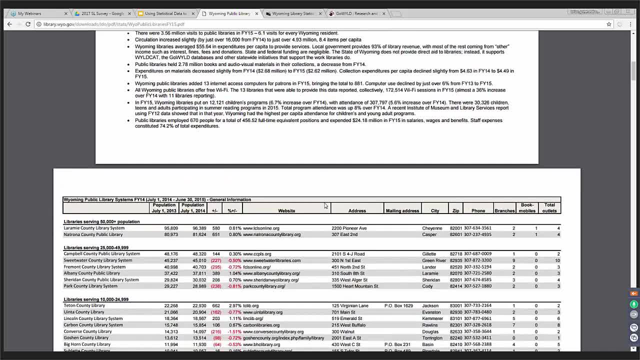 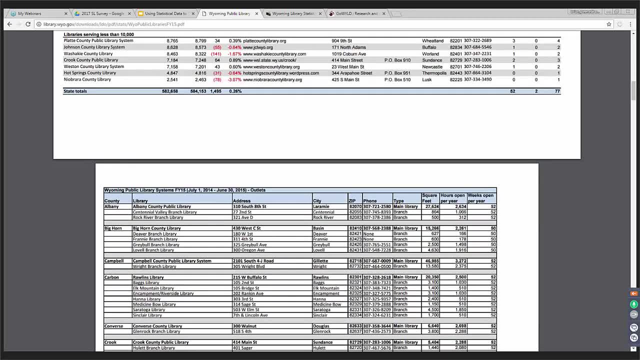 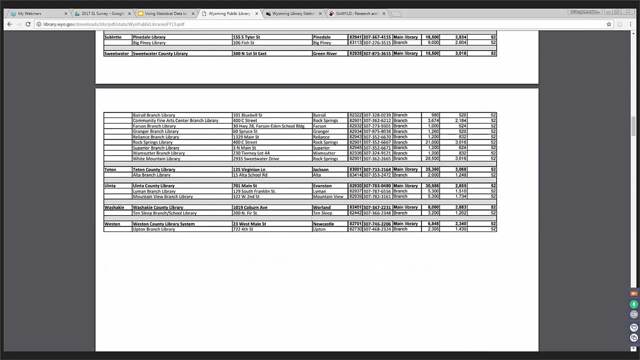 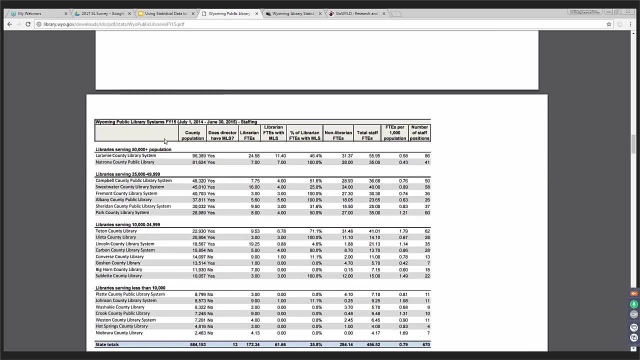 So utilize these and it'll make your life easier. We include about 15 pages of information from our raw data, from the survey, in this summary, and in some instances we give a little bit additional. like this one has to do with staffing. 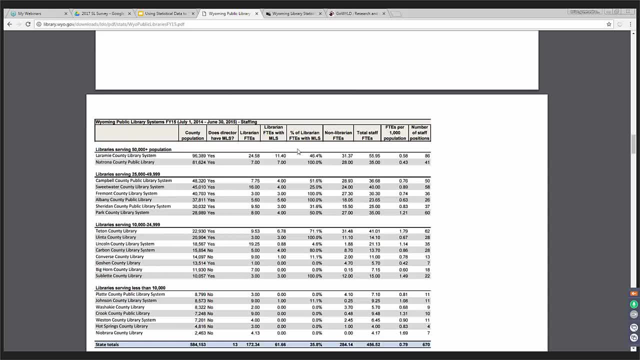 and the librarian FTEs with an MLS. well, we've varied out the percentage for you and then at the bottom are the totals for the state. So if you were any of these counties, you could compare it to the state total and see. 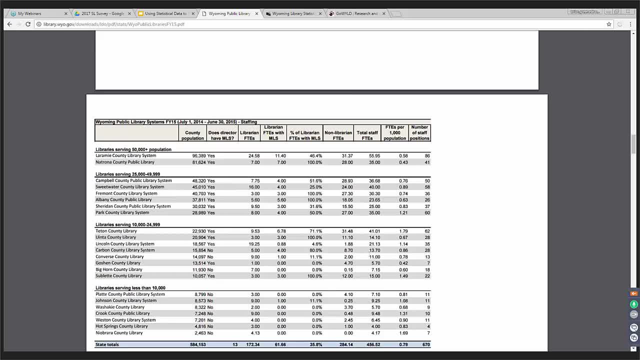 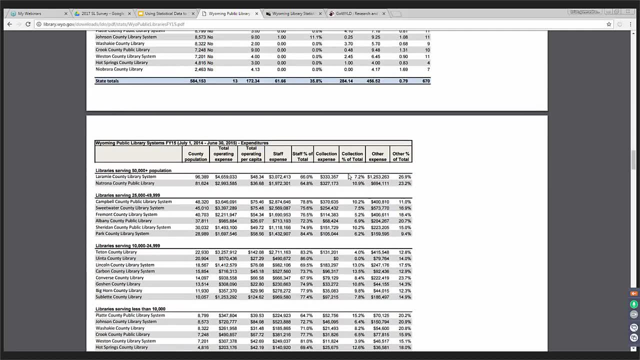 how your library fits in with that. overall. We don't do that for all of them, but we do for some of them, and like this one on expenditures, something useful would be the percentage, And the reason it's important to use the percentage is because sometimes you're looking apples. 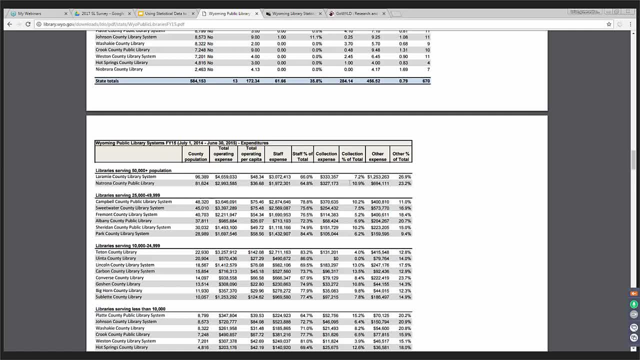 to oranges. it's a way you can. if you're a small library, you can compare yourself to a large library, Because if you look at the actual number it's going to be disproportionate, But if you look at the percentage, then it can still give you a comparison, a way to 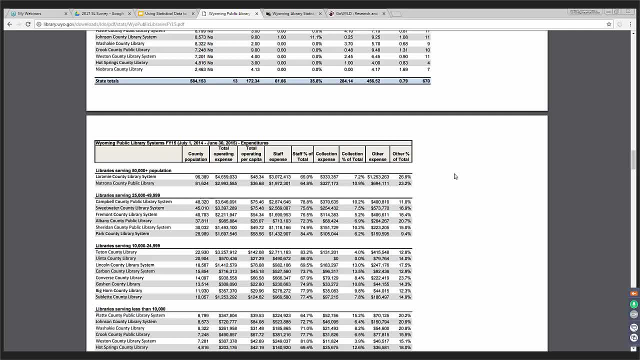 compare with those either large or small libraries, So you don't have to compare with all the libraries like yours, but we do break it down by community size for most of these, And so you could compare within your community Your community size as well. 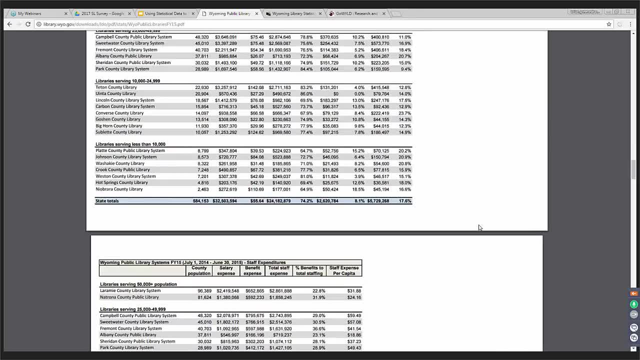 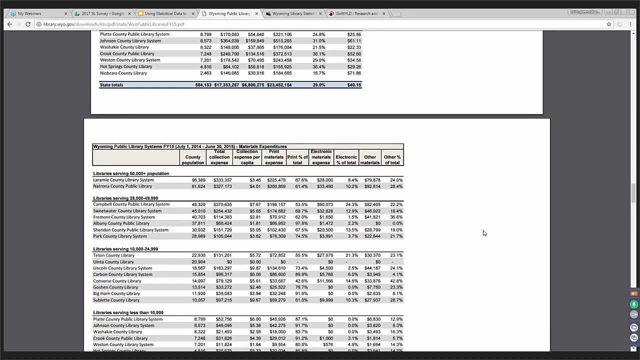 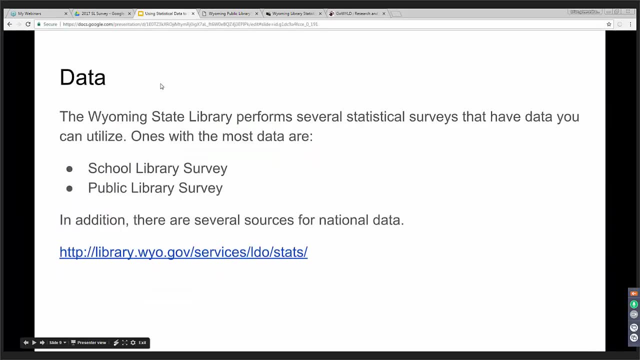 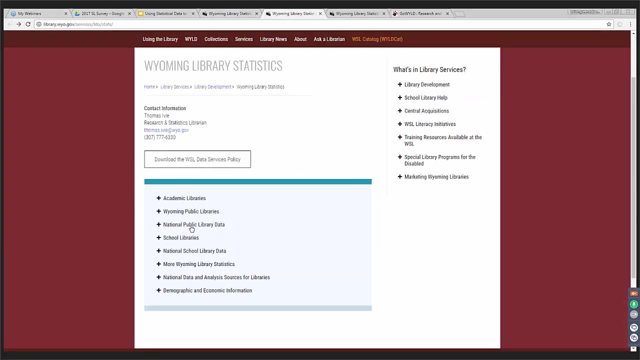 Let's see. we do the same with staff expenditures. So basically, we go through each and every portion of our category of our survey for that. There are also some national public library. Okay, Okay, Okay, Okay, Okay, Okay Okay. 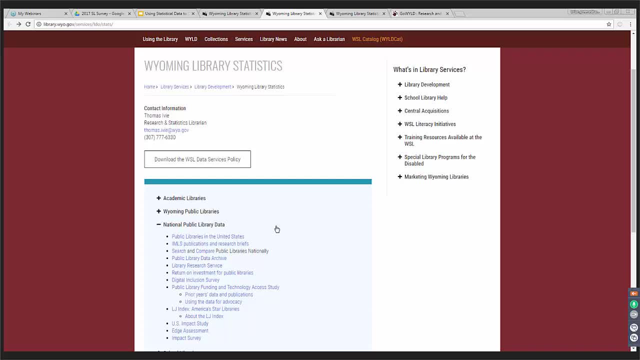 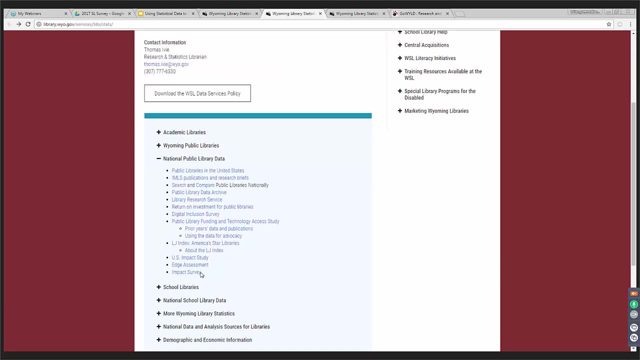 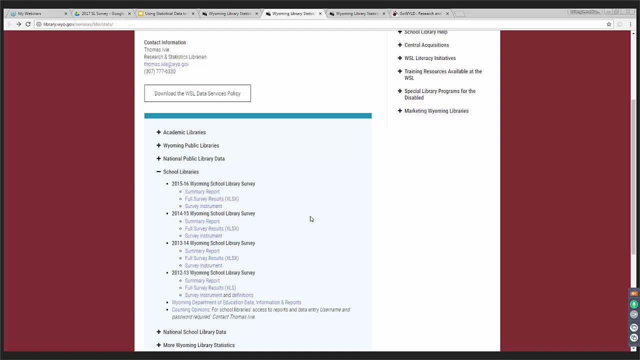 data And if you're doing comparisons, maybe on a national level or regional level, these might be useful. I will let Paige talk about the school libraries survey. Yes, The school libraries survey survey is also done every year and we have the latest set of data for 2015-16. 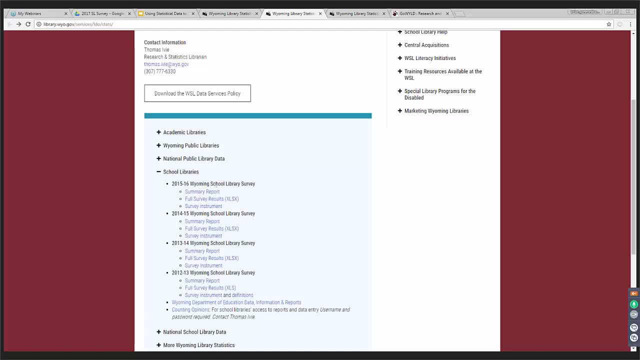 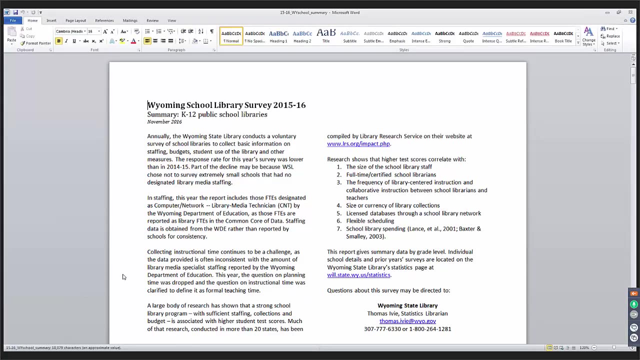 we are currently collecting data for 2016-17 and that will be posted this summer, but we offer summary reports. just like Thomas explained with the public library survey, we have taken the data and compiled it into statewide snapshots of different categories. so if you want to see how the state is doing, 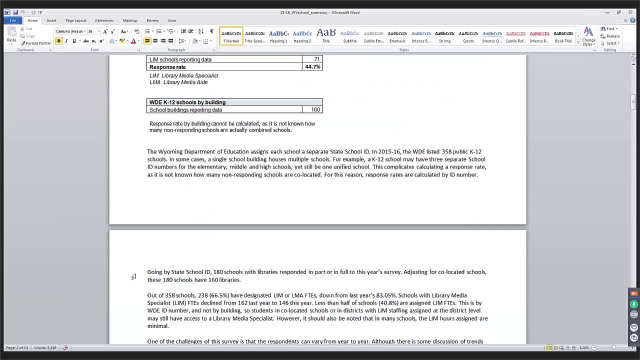 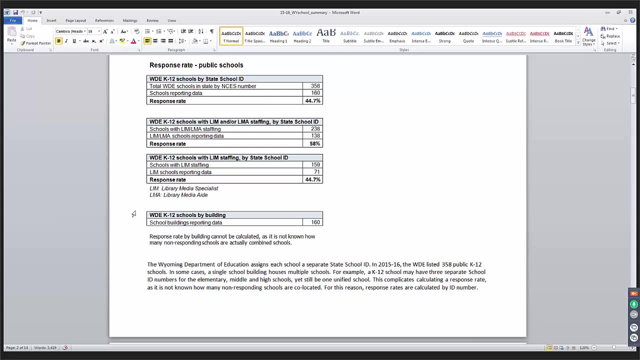 as far as staffing, or expenditures or collections. you can look at this and get an idea of what's going on across the state. the first sets of data that we come to, though, are numbers that are provided by the Wyoming Department of Education, and These are numbers that we cannot change. 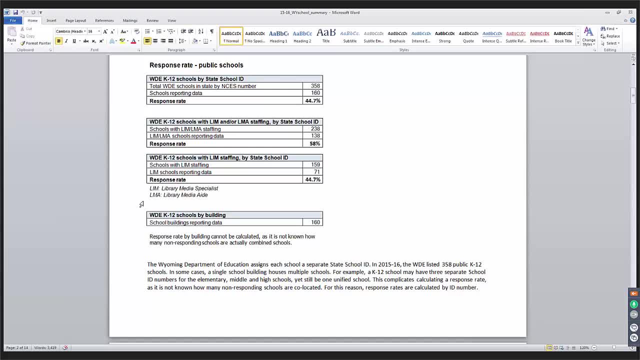 They are the enrollments, the number of schools and the number of library staff members throughout the state of Wyoming And these are reported by each district to the WDE. So we do start with these numbers and we have to stick with them. 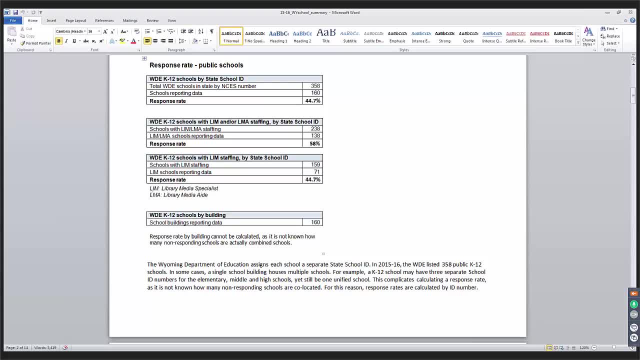 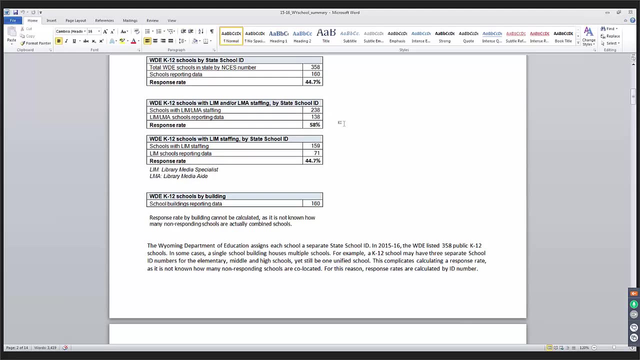 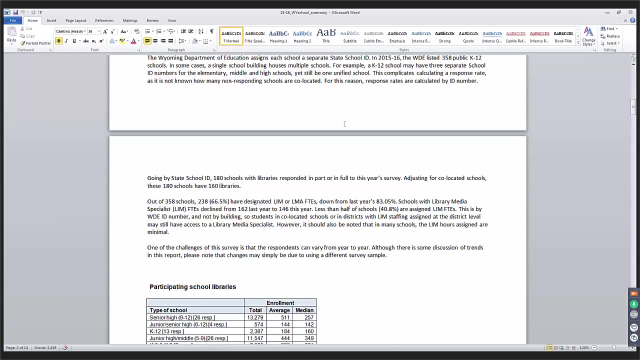 But this set of data also shows how many schools were reporting data for the 2015-16 school year, And out of 358 schools, we had 160 respond to the survey. But as you go down through the summary, there are paragraphs that help explain. 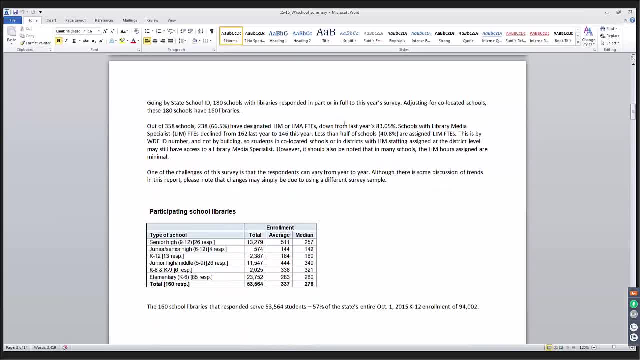 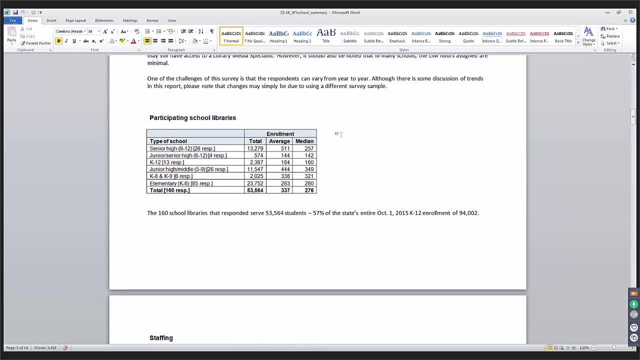 how this data can be used and what it means. And our schools are also broken up into different sections, For instance, senior high, which is we count senior high as nine through 12,. junior senior high- six through 12,. the K-12 schools, the junior high, middle schools. 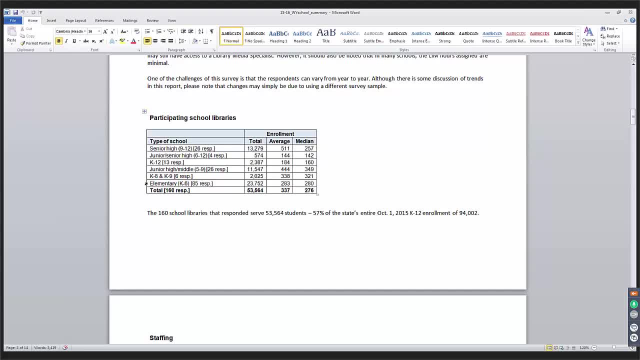 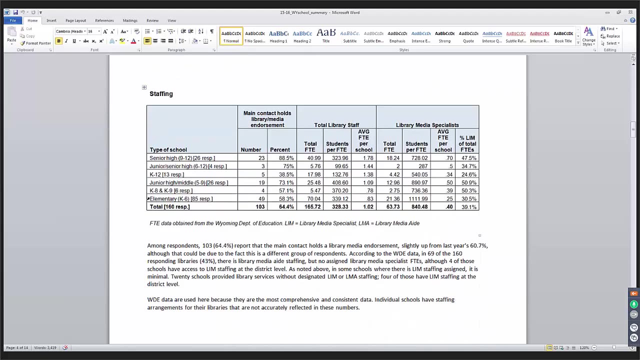 and so on down to elementary. This makes it a lot easier to compare your information. instead of comparing with the whole K-12 range. If you are an elementary school, then you can compare to other elementaries And then, as we go down through the different categories. 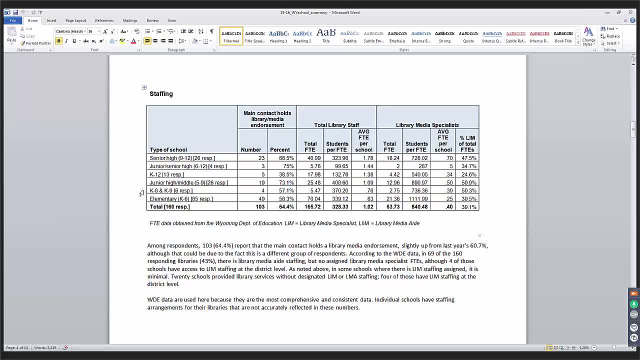 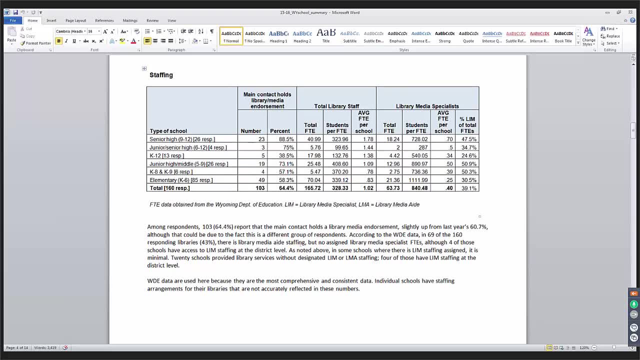 you can see how each of these grade level sections measure up as far as the different categories. And again, the summaries, the paragraphs, will explain what this data means. This is great if you want to compare your local data to the statewide, if you want to compare your data. 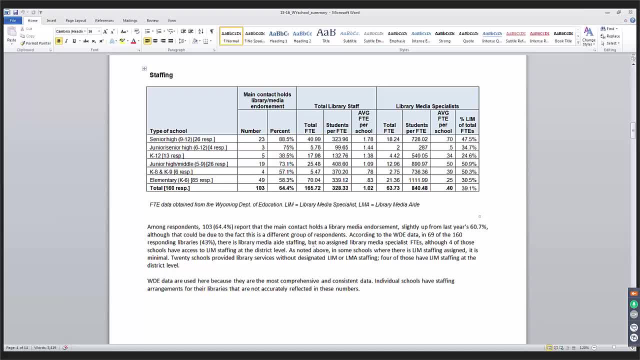 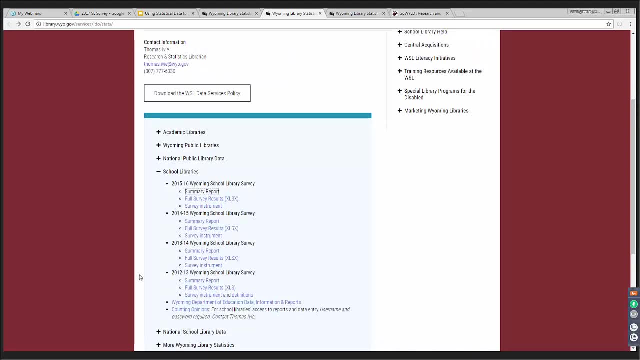 to similar size schools and grade levels. And it's also great if you just want a snapshot of the state of Wyoming school libraries. And I think something important about that school library survey is that that's the only form of, it's the only source of data for school libraries. 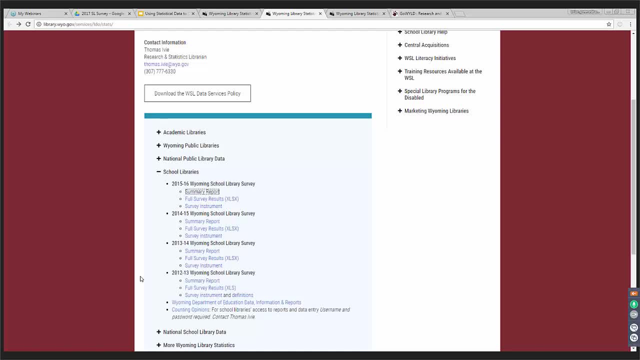 that we have in Wyoming, So it's important that schools do participate in that survey and complete it. That is a great point, Thomas, And on a national level, surveys and research is not being done on school libraries, And so this is about the only data, especially in Wyoming. 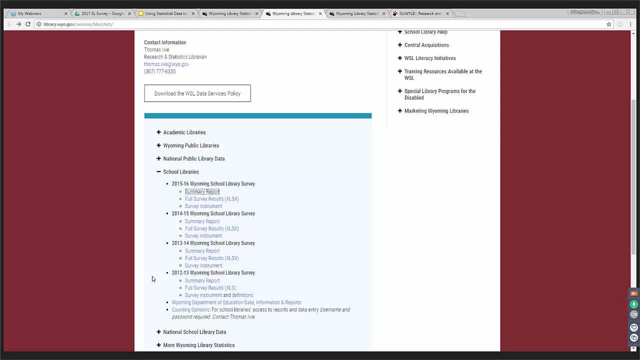 but not a lot of states do their own surveys. Some do, But it's really important to get this consistently collected data And the more schools that participate, the better able we are to see the state of school libraries. Also after the summary report, if you. 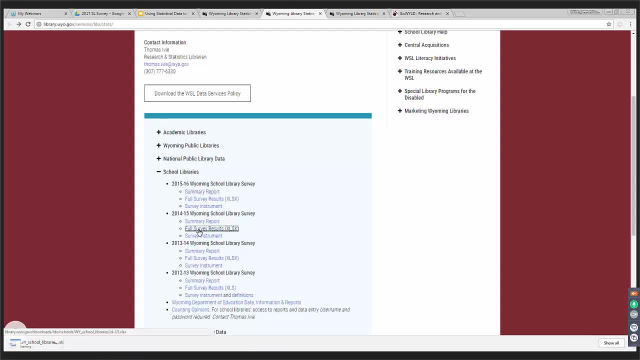 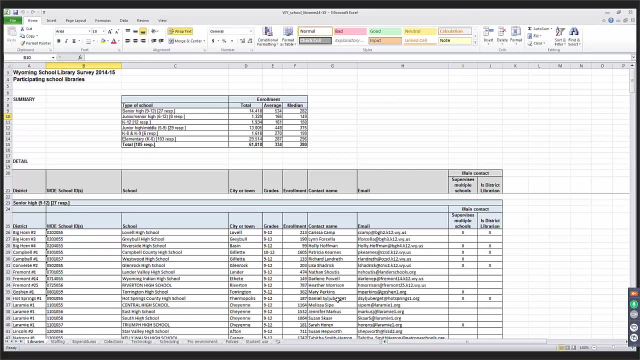 want to look at your own school's data after the summary report. if you want to look at your own school's data- schools data- we do have the spreadsheet. this is where it can be a little overwhelming, but we'll go through this here quickly in the spreadsheet there. 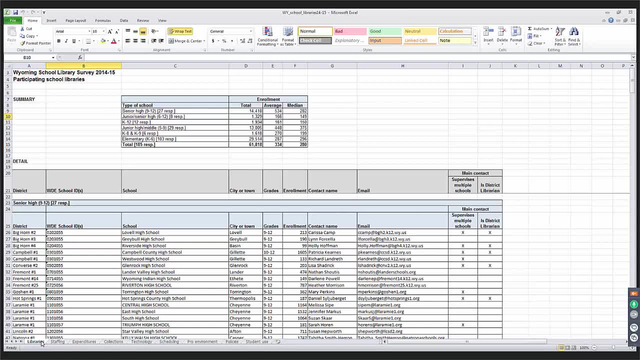 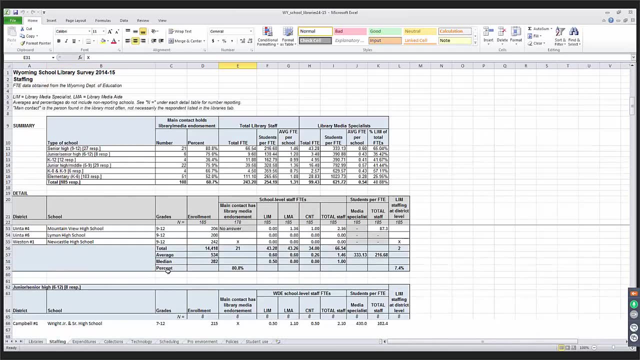 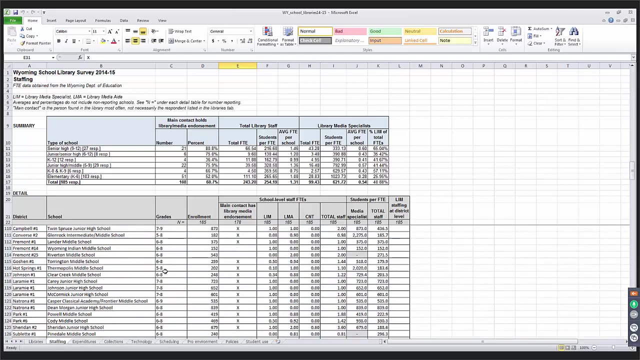 are different folders for the different categories. so, like here, we have the libraries. this is simply the libraries that have responded to the survey. we have the category for staffing and you scroll down and see the different grade level and sections that have responded, and then you can find your school and 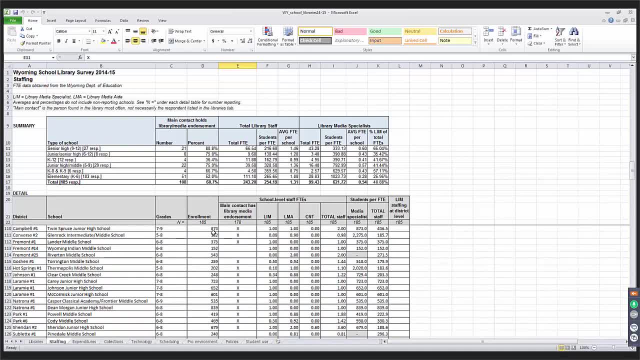 find the data you can. with the enrollment, you can compare according to similarly sized schools, you can compare data and you can go on through the different categories to find the categories that have responded to the survey, and then you can go on through the different categories to find the data you can. 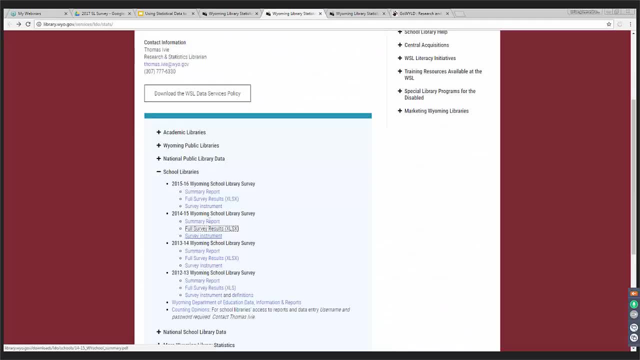 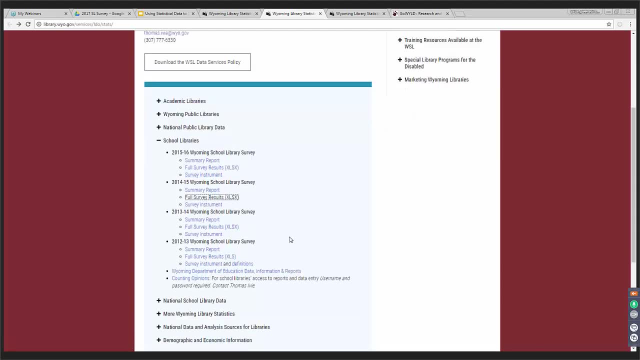 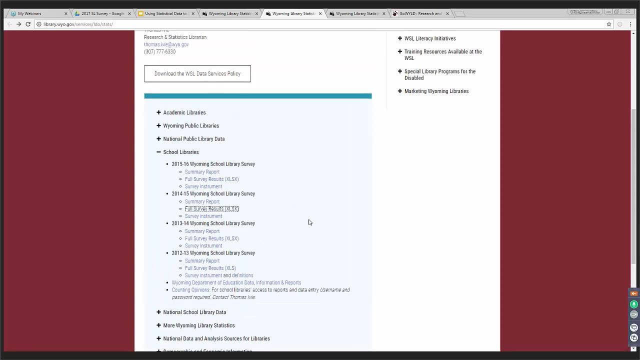 find the data that you're looking for. and then there's the survey instrument and that's the questions that were on the survey, if you want to get into that. and then the Wyoming Department of Education data, information and reports is also listed there. I'll turn this back over to Thomas to continue with different. 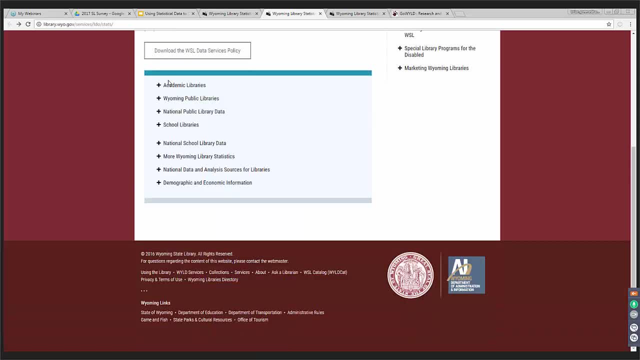 data sets. thank you, Paige. just as we had the National Public Library data, there's also National School Library data as well, so it's important to follow up with your state school library survey and in Wyoming, we encourage you to fill out the Wyoming one, absolutely, and you'll get a. 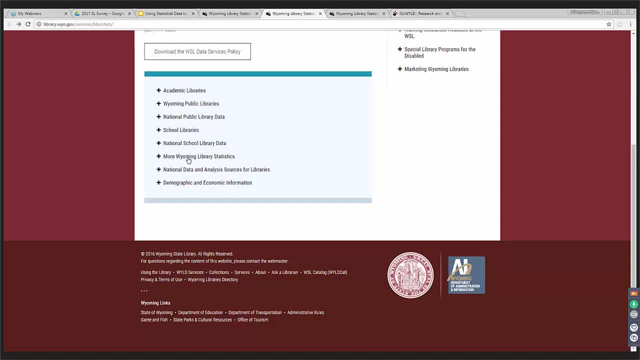 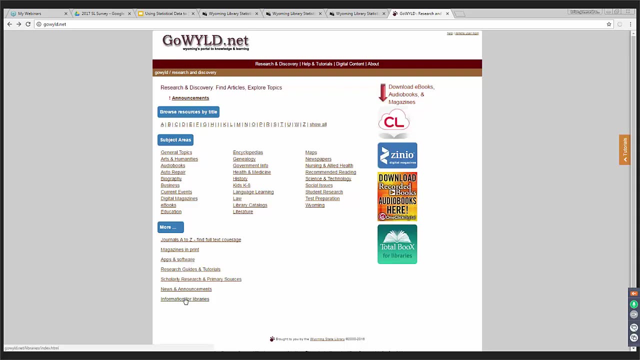 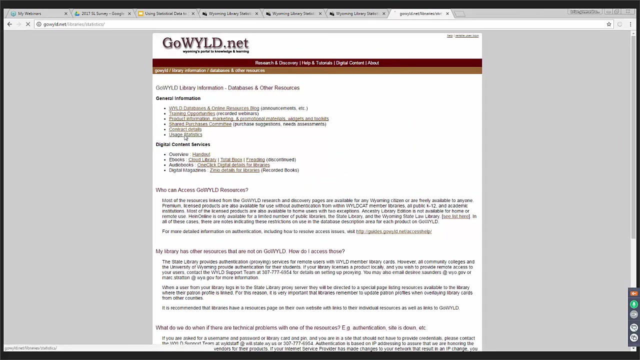 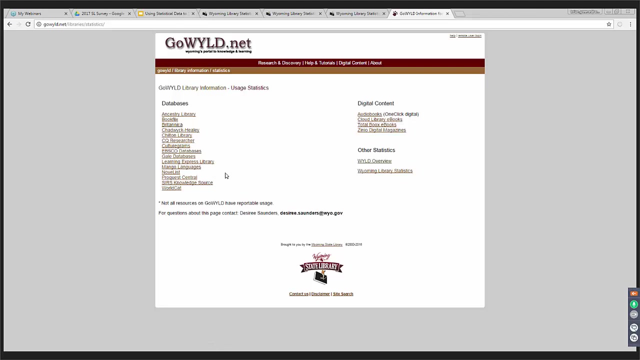 certificate. there's more statistics, and one that we would like to talk about is the go wild. if you're in Wyoming, a Wyoming library, you can see, you can click on more. and then we've got the usage statistics, and these are particularly good if you you know some. 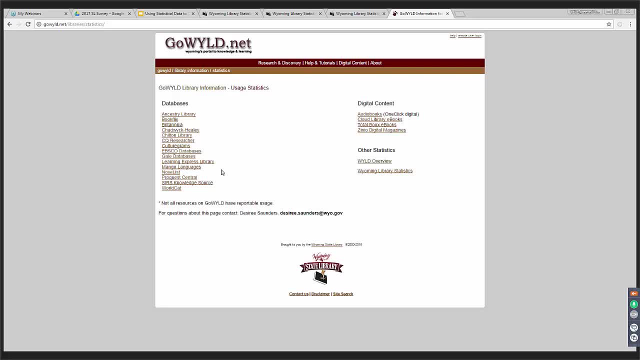 people don't know what they have access to, and they they're going to try and get some money for their budget too, for their school district, to buy some different databases so you can look and get a list of what's available, because these are available to all- all. 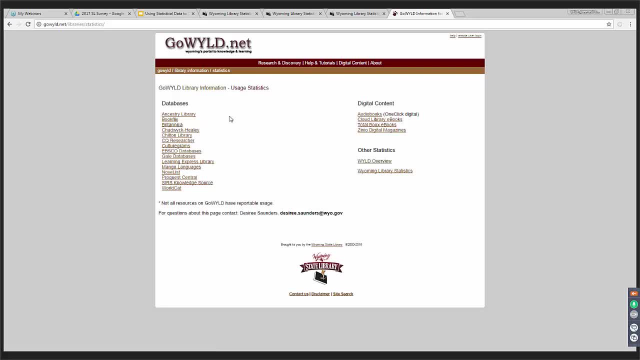 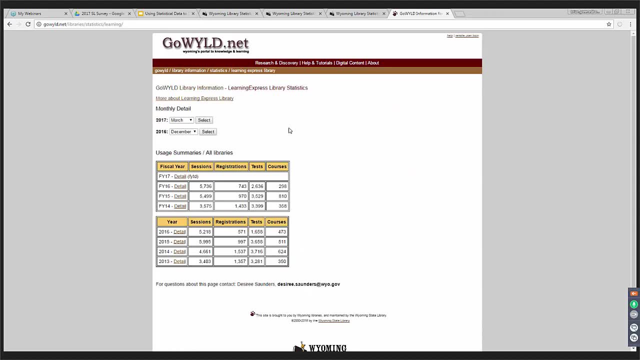 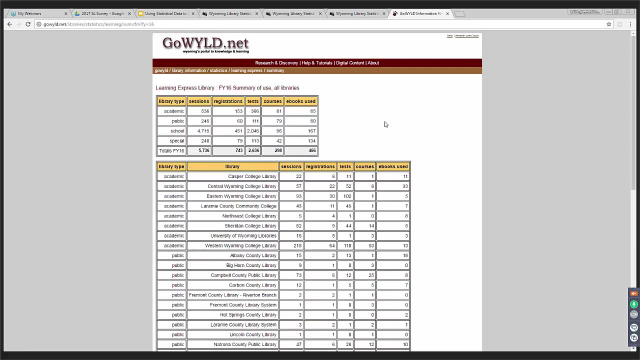 all schools, all residents and all residents. anybody in Wyoming has access to these and these usage statistics are great if you want to go in and see how much you use these databases are getting by your school district by. some of them offer detailed statistics and more information. there there are the concept ofے. 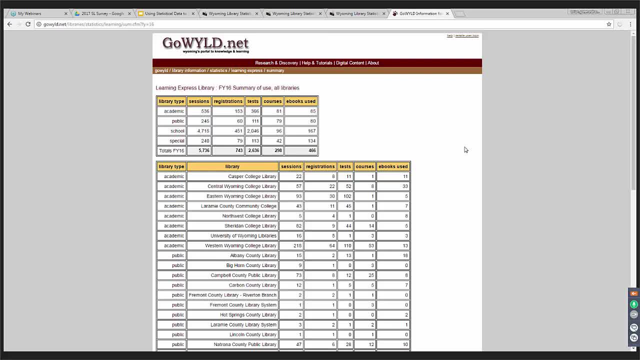 according to school. if you're at an academic library, you can see how much usage your college students or how much usage the databases are getting from your college students. public libraries also can find their usage statistics, and special libraries as well. these can be correlated to the data that is collected. 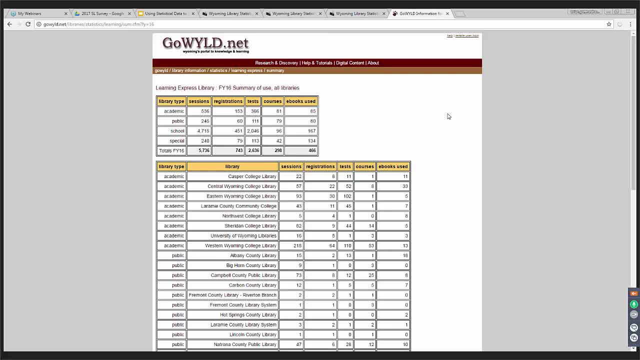 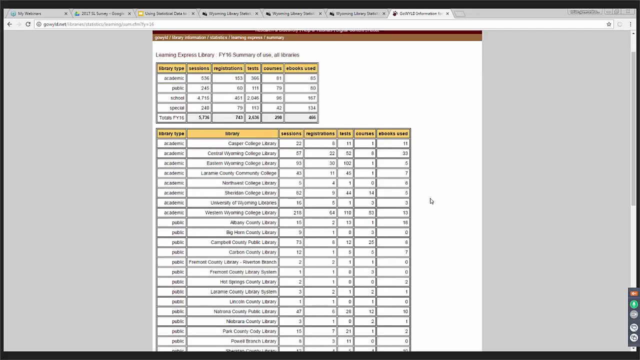 from the surveys and it gives a really nice snapshot of which databases in particular are being used by your community. so I clicked on learning Express library and you can see this broken down by academic public school. you can see if yours- you know if your school district- is on the list for. 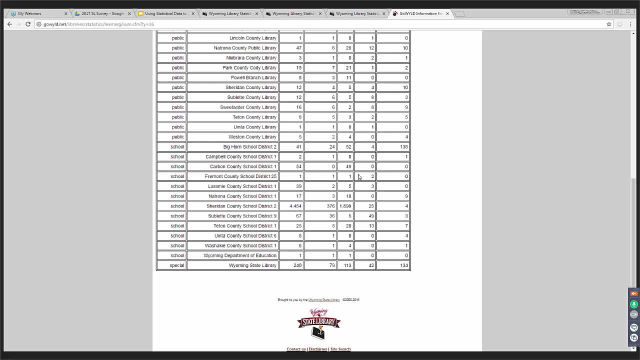 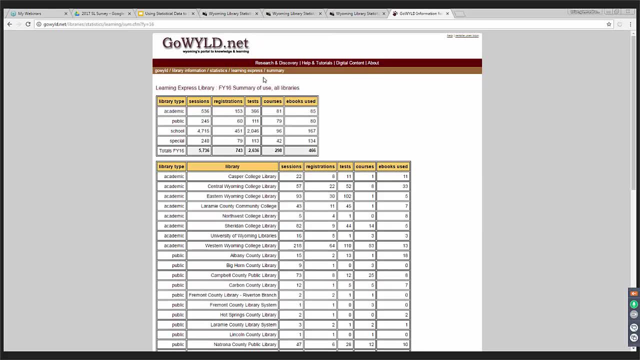 getting statistics for it, and you can use the any of these numbers from any of the database products for making your case. you can see the numbers for any of the database products for making your case and you can use the any of these numbers for making your case. 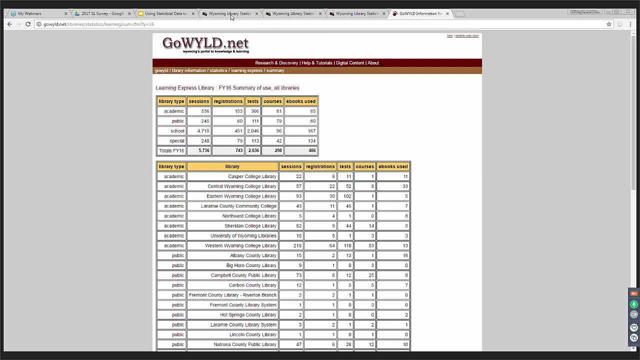 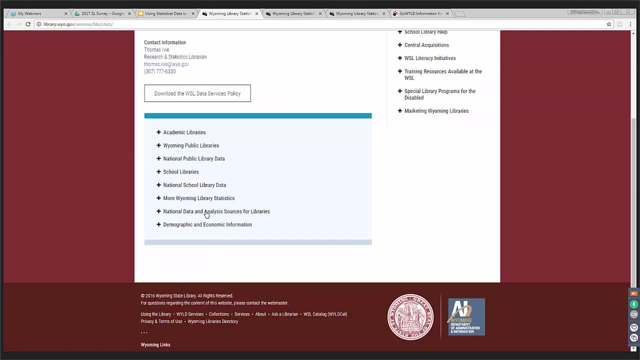 but we just wanted to show you that real quick so that you knew it was there. but we just wanted to show you that real quick so that you knew it was there. and then there's also national data, data and analysis. some of these are mentioned in some of the others. there's demographic and economic information, as 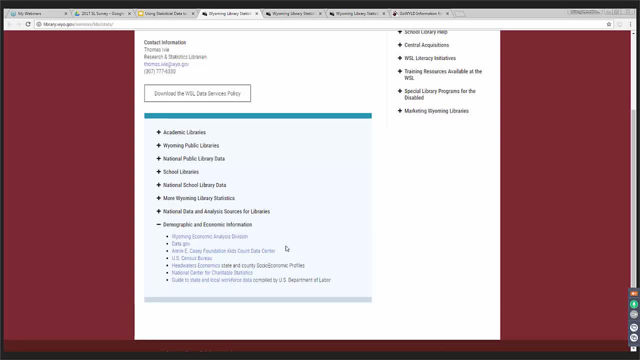 well. so if you need some big data for to present with, there are some sources here. there's also ton of other sources out there, so don't just let me know. if you need some big data for to present with, there are some sources out there, so don't just let me. 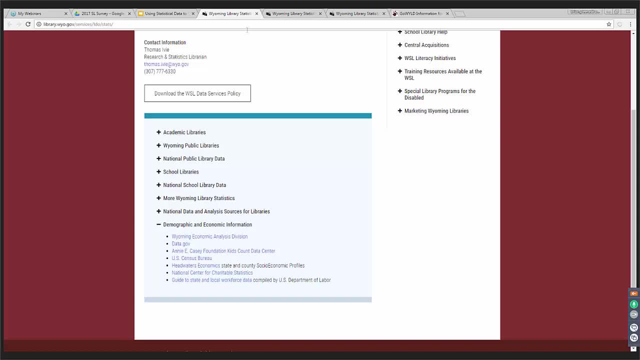 know. if you need some big data for to present with. there are some sources out there, so don't just let me know. if you need some big data for to present with, there are some sources out there, so don't just let me know if you need some big data for to present with. 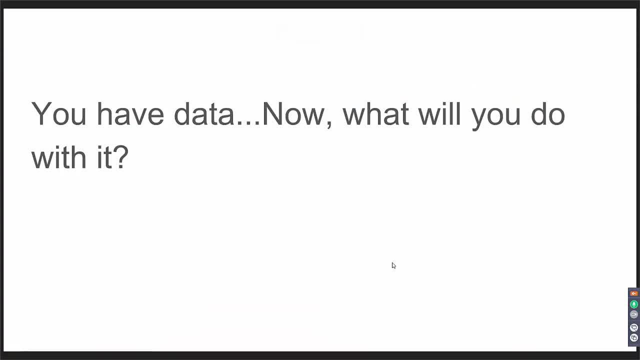 so you have data now. what will you do with it? data is important only if it. so you have data now. what will you do with it? data is important only if it gets used, and if data is collected but not analyzed, then it isn't helping your gets used, and if data is collected but not analyzed, then it isn't helping your. 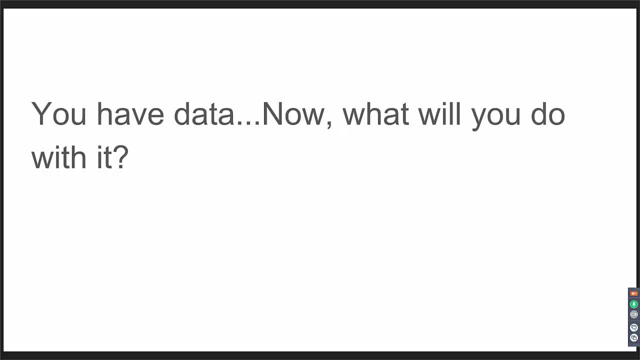 organization data can be a critical part of your organization if you know organization data can be a critical part of your organization if you know organization data can be a critical part of your organization if you know how to use it. looking at the data without knowing the story you want to tell can be an overwhelming task. So take 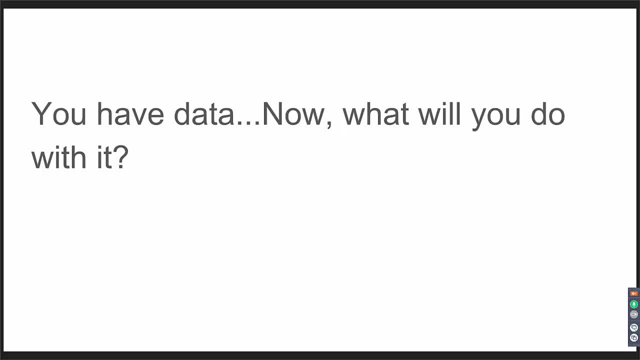 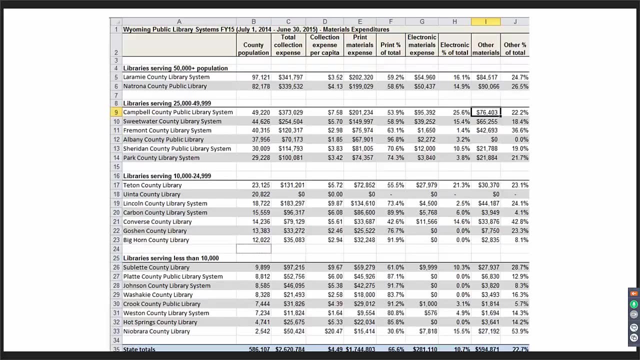 a look at the data and take the time to analyze it and shape it. Find the data you want that's going to help you tell the story that you want to tell. You will want to isolate the data you want to use in order to tell your story. The 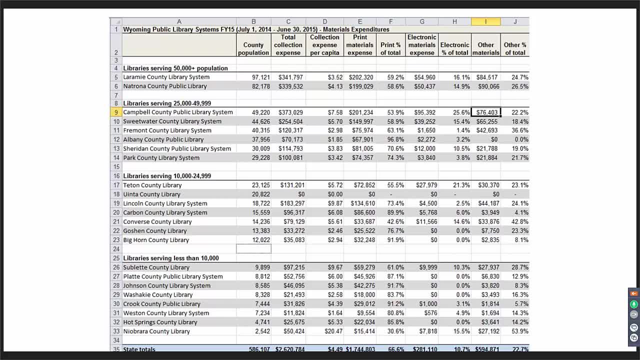 Wyoming Public Library survey has about 14 pages, as I said before, of data and that can be a lot to go through. So let's say we want to tell the story of what a library spends on their materials and this part of that- 14 pages of data. 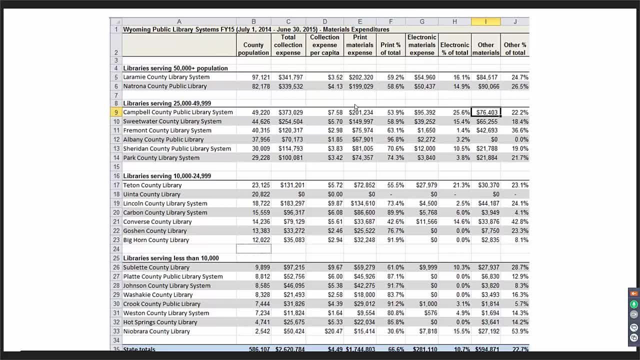 is one of the pages that has that: materials expenses. By taking the time to look through that data, we're able to find the correct data that we want to use to present. In this instance, we could just use the data for our own library, so whatever library you're from, 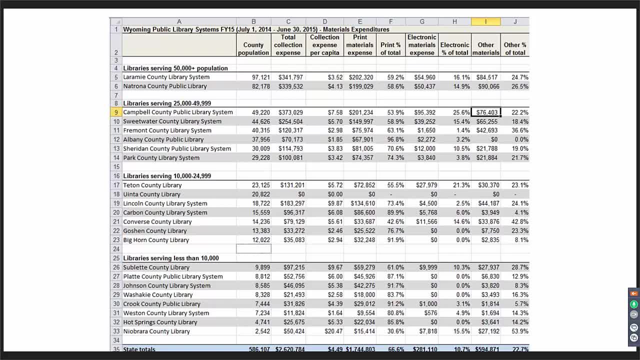 or you can make comparisons to other libraries with similar county populations or, say, total collection expense. You might even do it utilizing one of the other pages where it mentions what your budget is, So you could compare libraries that have a similar budget to yours as well. So here, 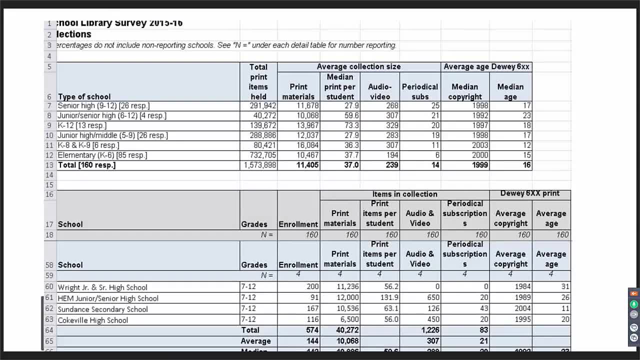 is some data from the school library survey. Let's say you are one of these four schools down here towards the bottom and you wanted to make the case to purchase a new science and technology collection for your school. From looking at this data you can make a strong case to. 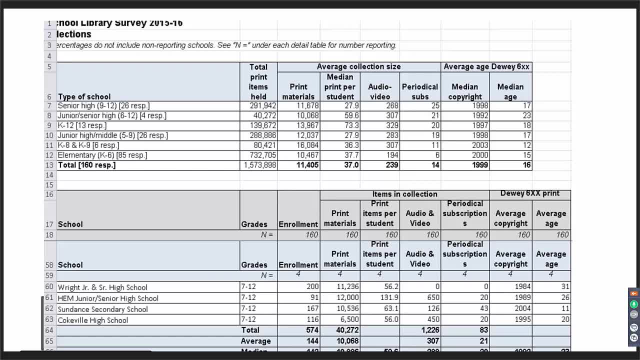 update the collection, since the average copyright date for any of them is so far out of date. Even if you have the most current copyright date of the school, the 2004,, it's still 13 years out of date, So it would make sense to use. 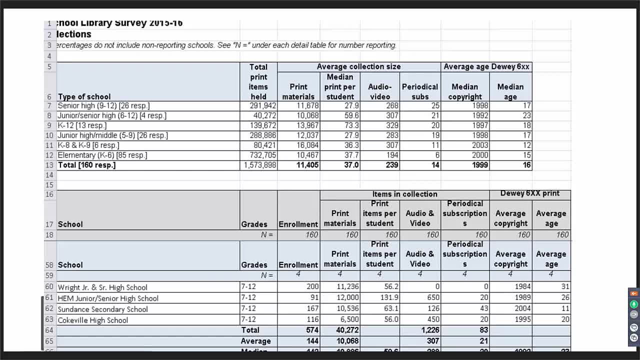 your school's numbers to try and convince administrators that your collection is outdated, because for the science and technology section to be that old, that's pretty well out of date And it's important to note that we've done some of the work for you. The total if you look up above it: 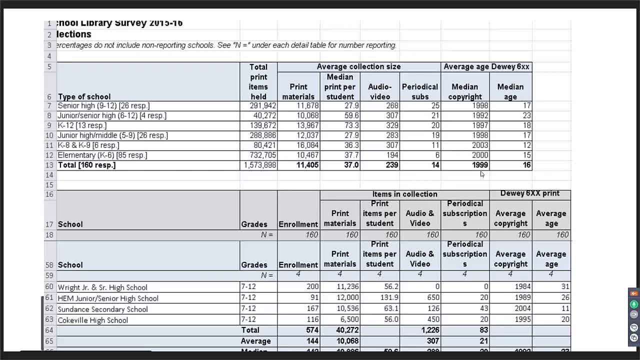 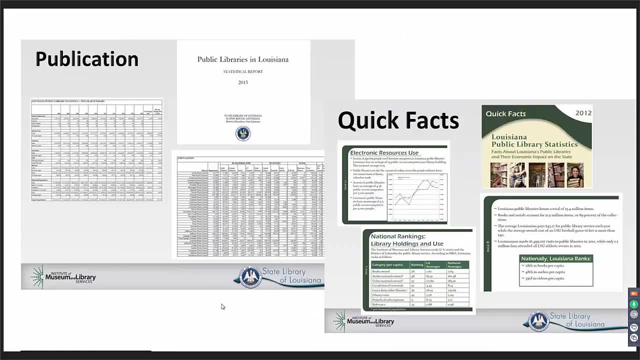 the other data, the average copyright date for that collection is 1999.. Wow, so not even in this millennium. Yeah, So you can use these things to make your case. The Louisiana State Library creates an annual statistical report and a quick facts publication which is much like the Wyoming State Library's summary. 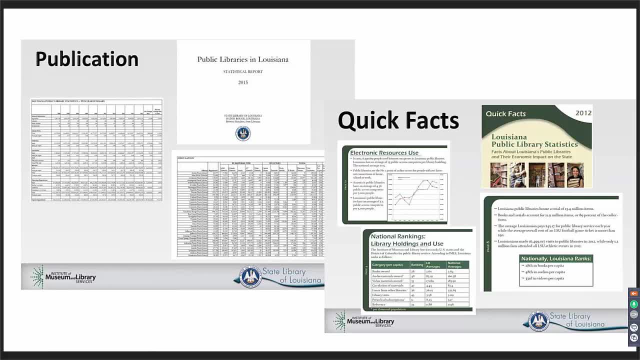 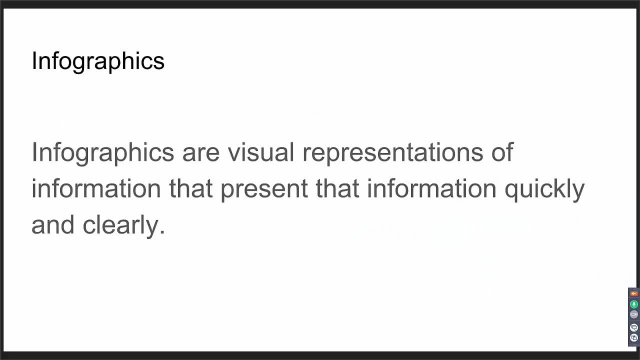 report for their public library survey. Most states produce these and they can be a great source of data for you to use because they give you quick summaries. Absolutely, Once we know the story that we want to tell and have the data to support our story, we need a way to communicate it to the audience- Audiences. 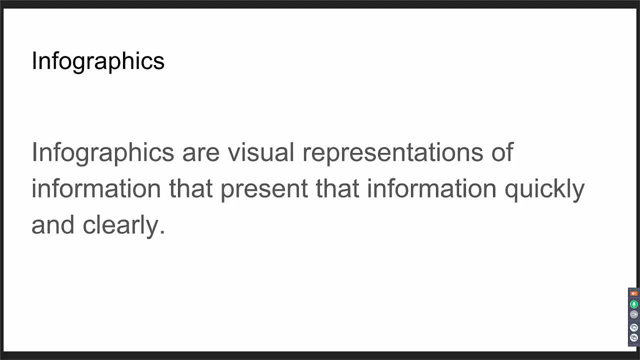 differ. They can be boards, county officials, principals, superintendents, the public, anybody. With any of these audiences, you want to present the information quickly and clearly. While there are many ways to do that, infographics deliver the story of. 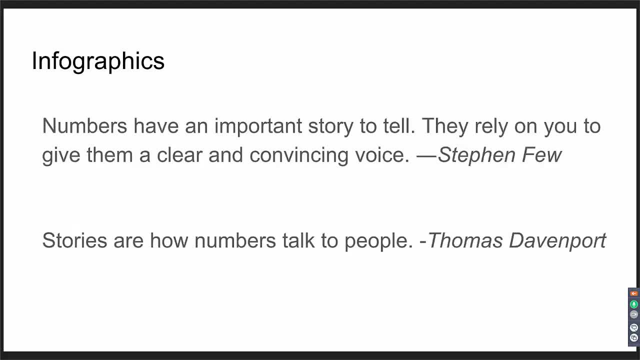 the data in a concise way. Here we have a couple of quotes on telling your story, One by Stephen Few: numbers have an important story to tell. They rely on you to give them a clear and convincing voice. And then another one by Thomas. 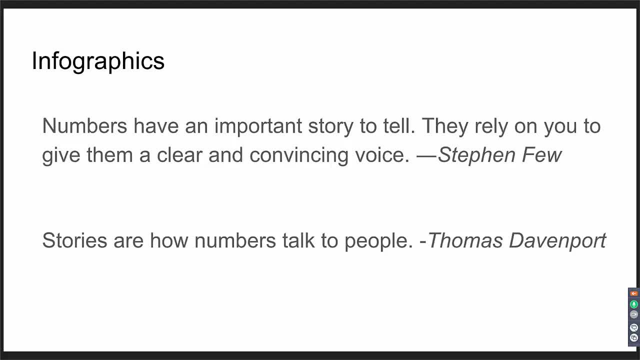 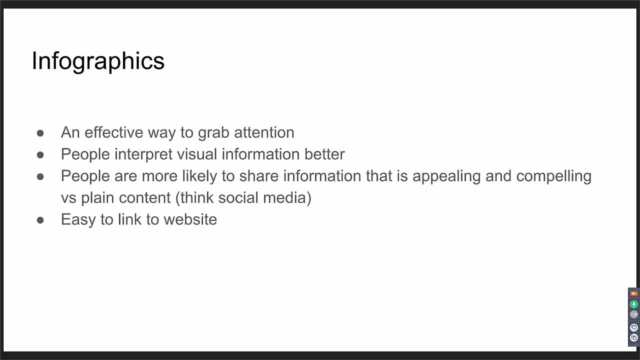 Davenport. I'm going to start by saying that stories are how numbers talk to people. Infographics have emerged as one of the most popular and sharable forms of social content because they are effective, they make it easier to interpret the data, they're easy to link to a website and people like to share visually appealing. 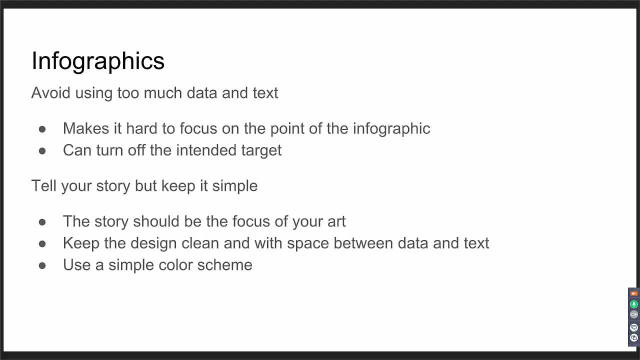 data, But your story can get lost if you use too much data. Viewers should be able to understand the information presented in a single reading and to use it to single reading, So using a theme of graphics that relates to the subject of your story. 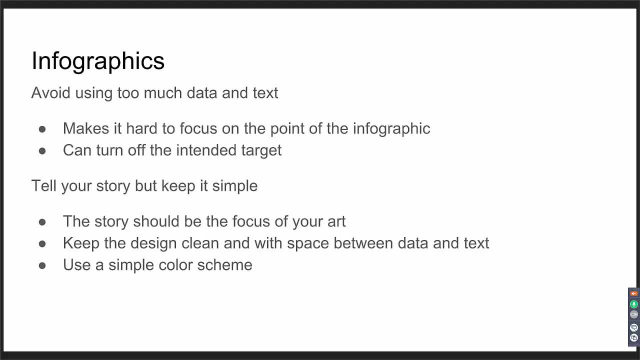 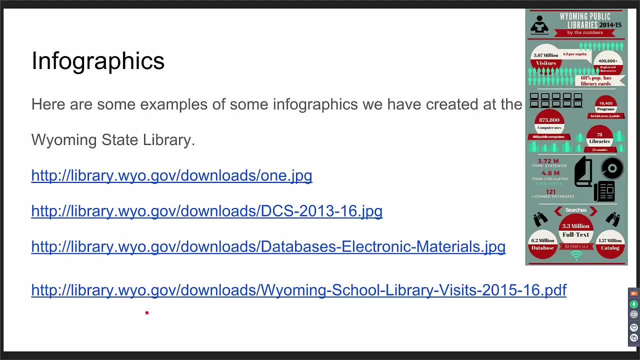 can increase the viewer's attention to the infographic. It is also helpful to use space between the data and text in order to keep the focus of the story for the viewer, as does using simple color schemes Alright. so here we have some examples of some infographics. 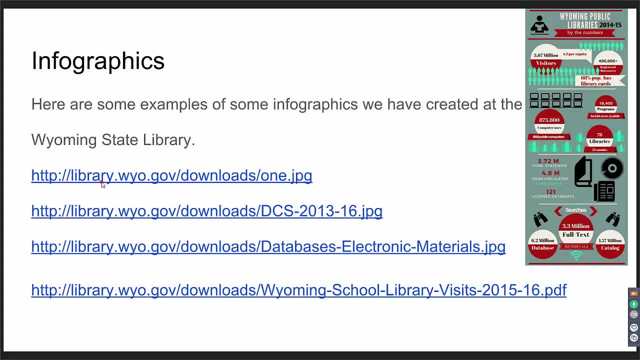 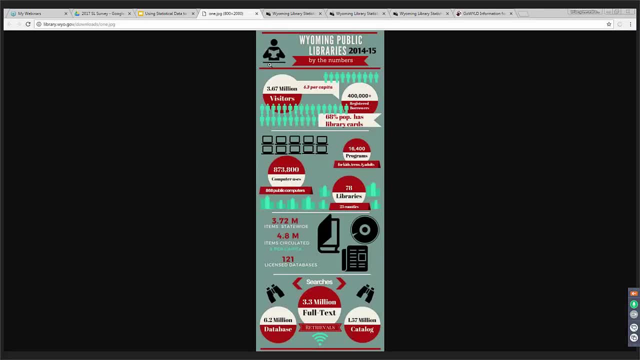 that we've created at the Wyoming State Library. I'll click on them and talk about them. This first one here has to do with the library statewide. We took this information from the Public Library Statistics- the 2014-15, and we tried to utilize- you know- open space. 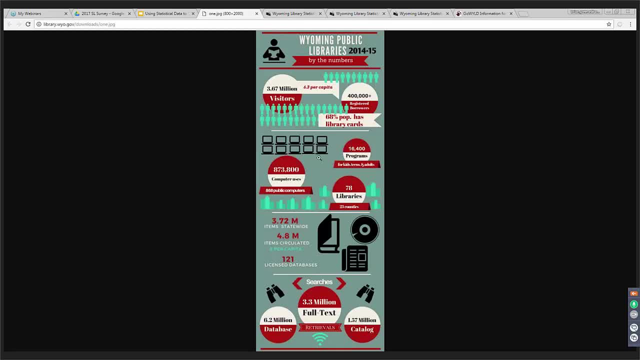 and some graphics, but not get overly complicated with it, Mostly just giving numbers, And we broke it down into sections. So the first section is: you know how many visitors we had and how many registered borrowers, what percentage of the population has library cards, And in the next section we had the number of computer. 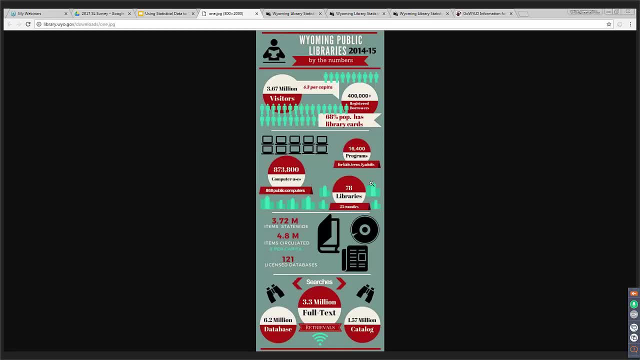 uses, number of programs and the number of libraries that we have throughout the state. And then items circulated, our licensed databases, how many items there are statewide, as well as because databases get a lot of hits, You know you usually have large numbers there. 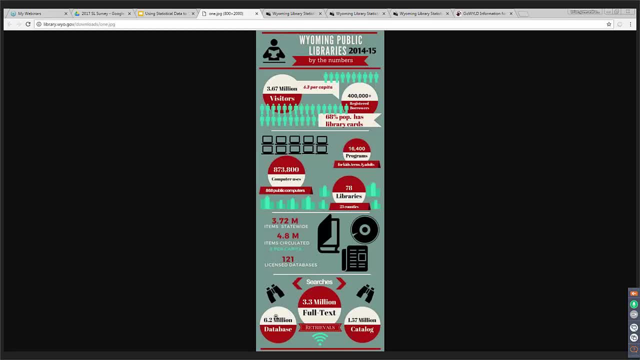 And our numbers. we have 6.2 million uses of the databases, 3.3 million full-text retrievals and the library card. the statewide library catalog had 1.37 million or 5.7 million- sorry, hits on it. 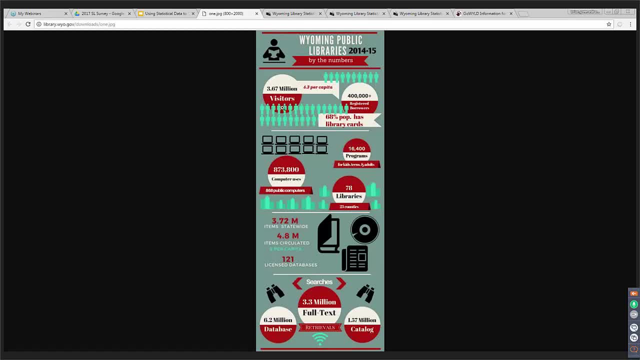 And while these numbers up here- the number of visitors and the number of registered users- may not seem large to outside states, those are pretty good for Wyoming, You have to remember. Wyoming has the lowest population of all the states. So we like to use this percentage of the population that has library cards because then we can compare ourselves to other states. 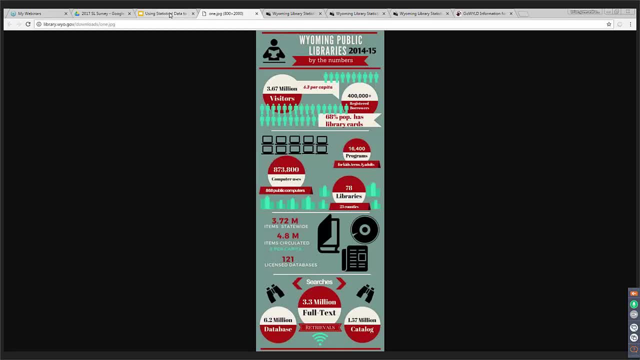 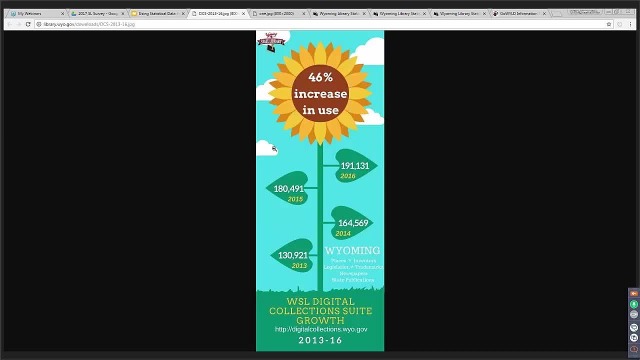 and see how we're doing, We'll go to the next one. We created this one to provide information on our in-house homegrown digital collection suite, which we thought was important, to put what those products are down here and then to provide a website for readers. 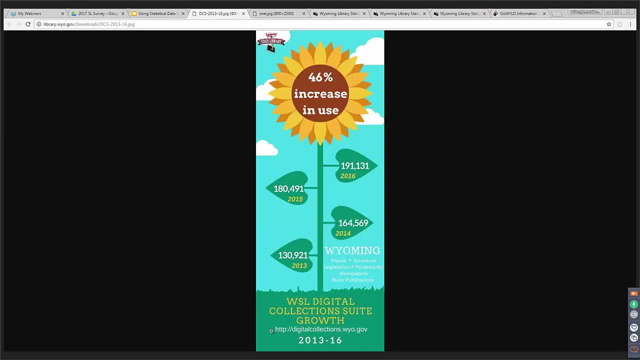 So the first thing we did is we created a website for others to see if they wanted to write it down or when they see it so they can go to it, And the information we wanted to portray is how much it's grown over the course of four years. 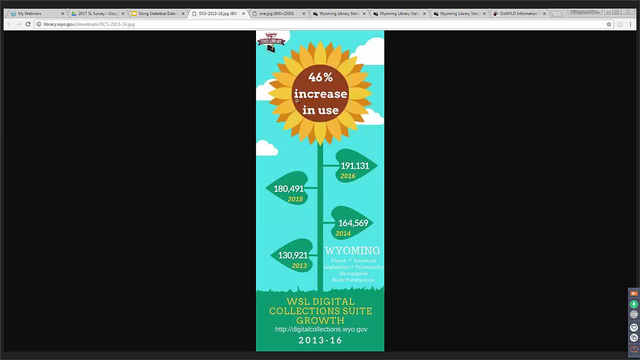 So 2013 to 2016,. it's grown a total of 46%. Part of infographics is choosing the appropriate graphic to portray your information. and sunflowers grow pretty fast. And the thing is about. six months ago there was a lot ofited information for vendors in the state of Wyoming. 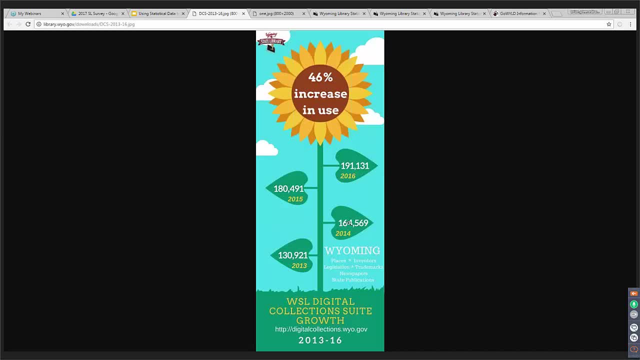 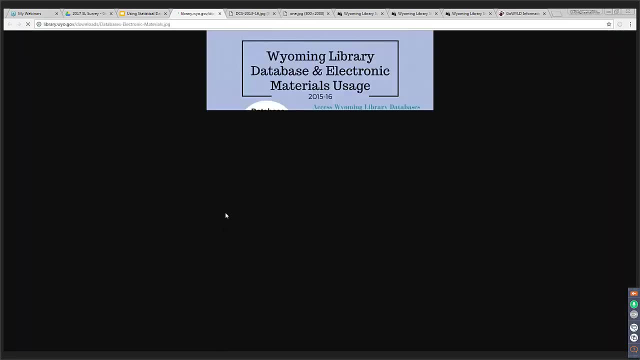 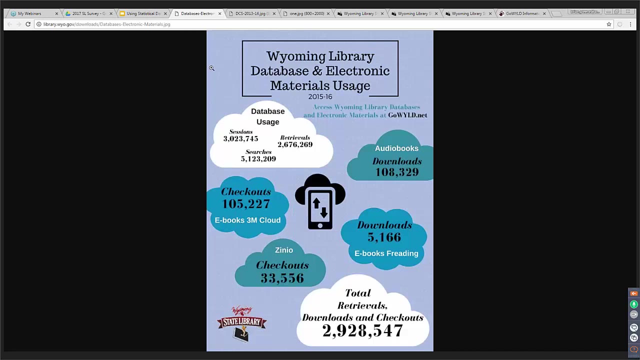 But we didn't know that they were going to grow anymore pretty quick, and so we thought that would be a good one to use this next one. we wanted to provide information on the database and electronic materials usage, so we chose to use a. you know different clouds to put the information into which. 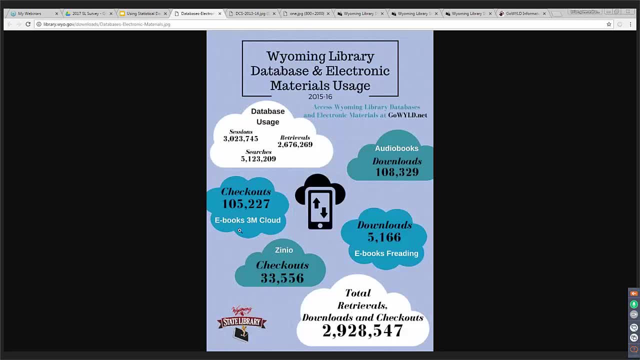 we didn't want to provide too too many numbers, because if you have too much information it can get lost. but we still provided the web address that they can go to to access audiobooks and ebooks and the online magazines. and then we try not to use too many colors. we tried to kind of stay in a sort of a color scheme, just 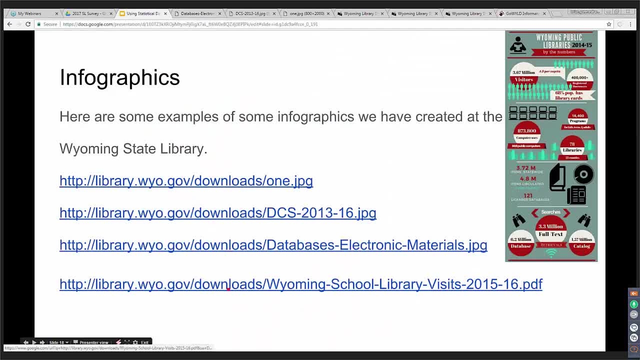 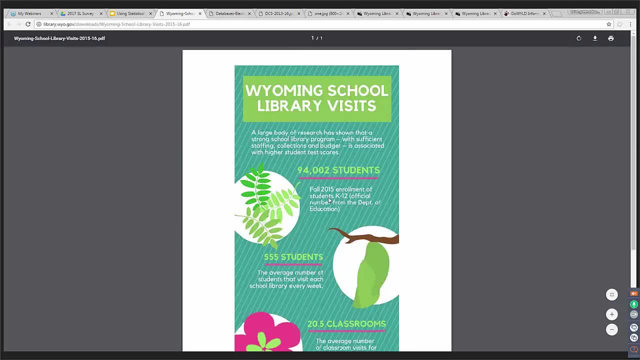 trying to keep it simple. and then this last one I will let Paige talk about. it's on the school library visits. yeah, this is information taken from the fall enrollment, fall 2015, and the number itself. again, the enrollment was taken from the Wyoming Department of Education. 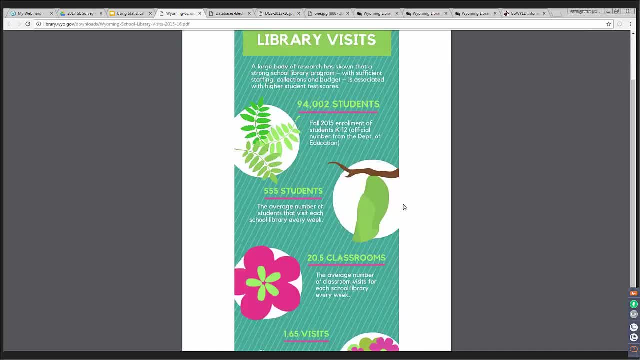 but the survey that we send out collects the data about how many students visit the note, visit the library, how many classroom visits there are, and so we took that information and compiled it into this infographic showing how many students, out of 94,000 students, what was the average number of students? 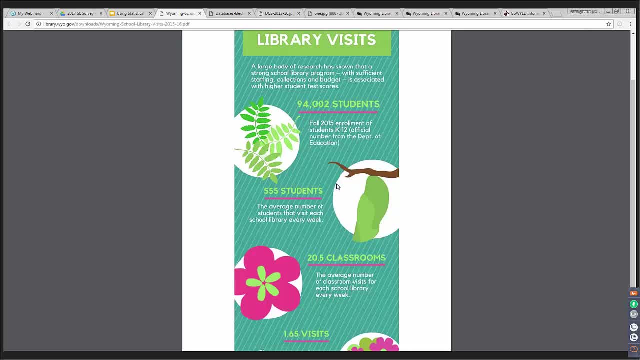 that visited their school library each week, and thus the data was reported as five hundred and fifty. a hundred nine hundred and fifty a hundred thousand students, in totalmente five THEY WERE WAS THE les of students that visited their school library each week, and the data was reported as five hundred and fifty. 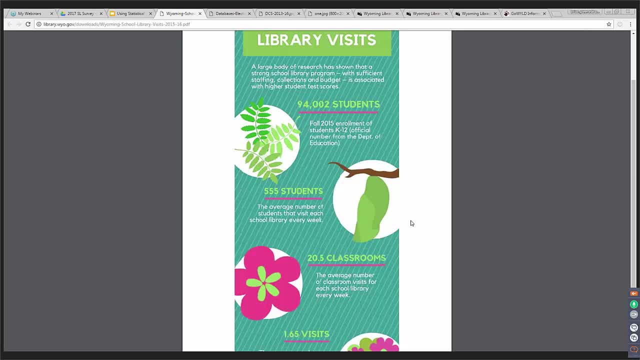 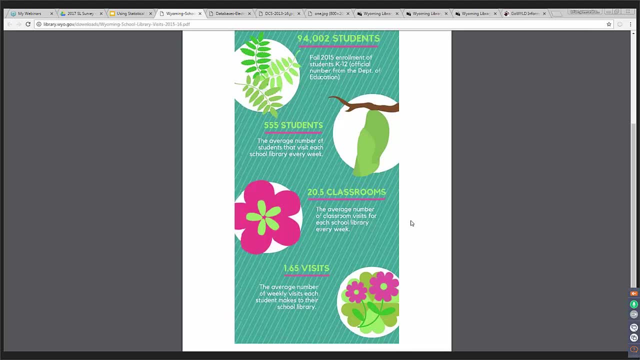 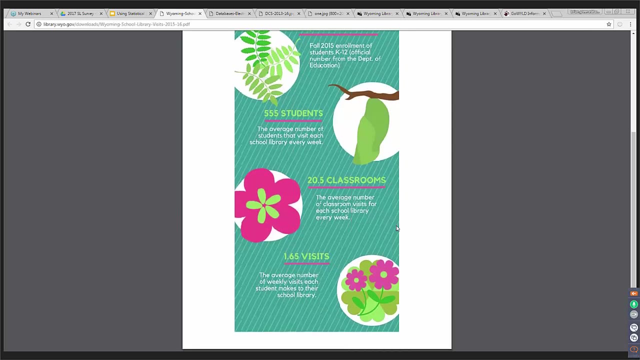 students visiting, or was the average number of students that visited their school library each week and the average number of classroom visits was 20.5 classroom visits a week to each school library, and then we had the average number of weekly visits each student makes, so each student according to the 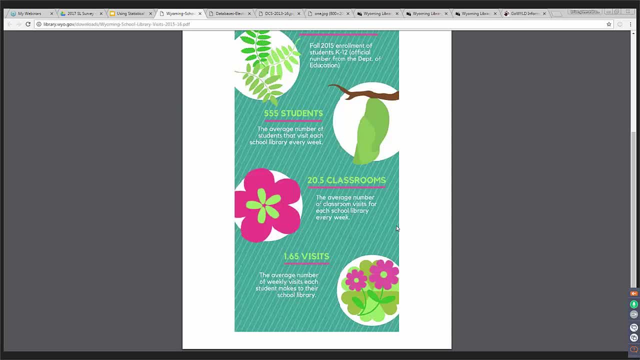 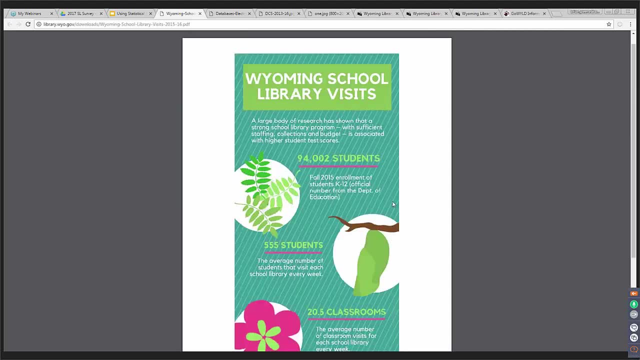 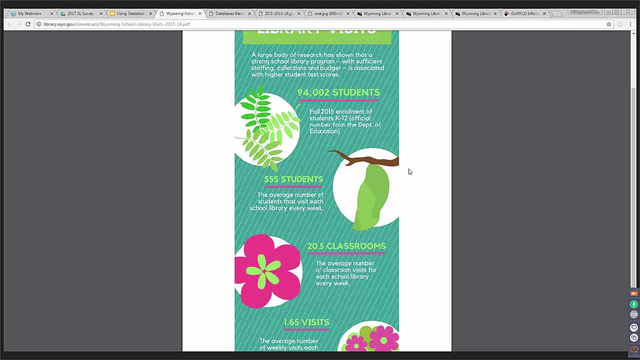 statistic, each student made 1.6- 5 visits to their school library each week. this is just a snapshot of one small portion of the data that was collected from the school library survey. as you can see, it's not a lot of information, just a few tidbits. and it's visually appealing: the colors are attractive and 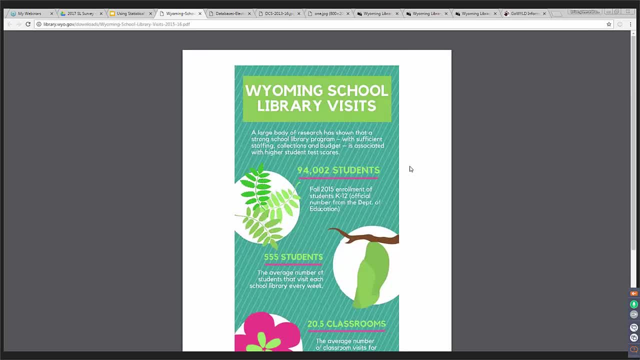 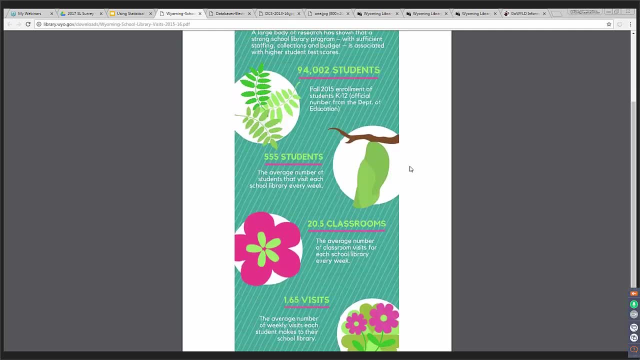 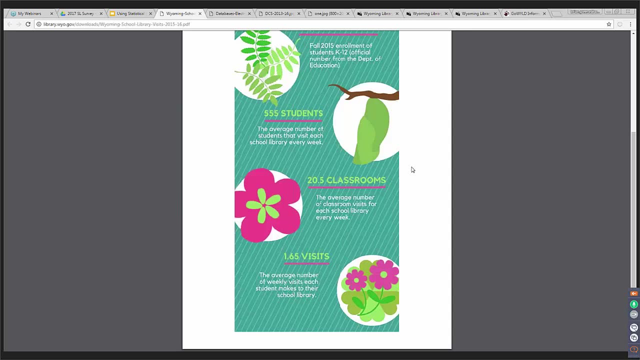 its latest out with enough space between the different tidbits of information that it makes it actually easy to read, and it's a nice infographic to just put up in your library to to send home with with your students, for parents to view, for your principal to see. you can also do this with your local data, with your 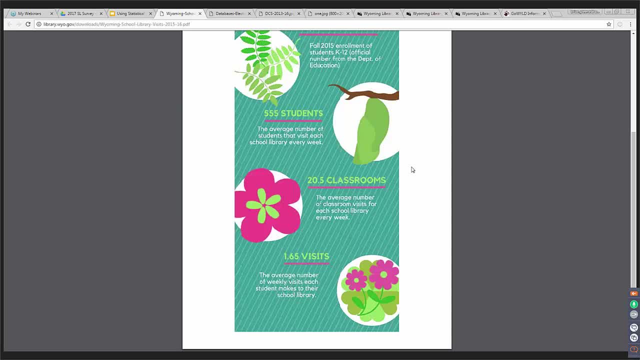 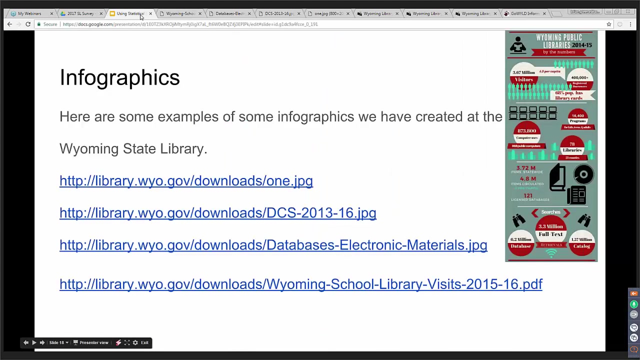 school data with your district data, and you can pull things like this and just make fun infographics that highlight one particular piece of data about your library, and you can even change that up and each week have a new infographic or a new factoid for display for people to see. those are the few examples that we 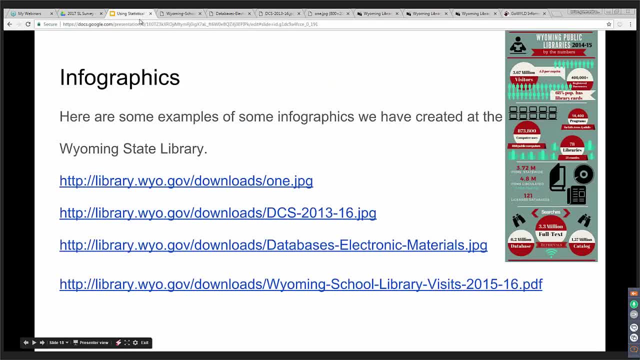 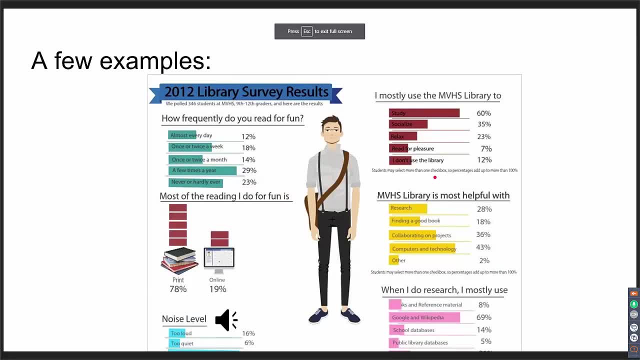 have. we're hoping that those give you some ideas, you and we're going to give you a few other examples here. so here is a survey of 9th through 12th graders about the use of their school library and notice the use of color in the survey and the student. there is a graphic of a student. 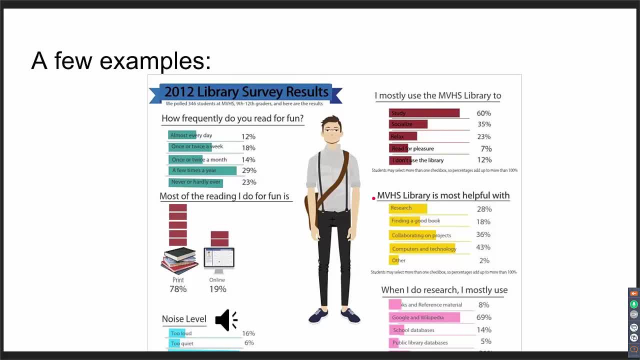 to indicate that this is data on students and it's interesting information. a lot of people would be would be interested to find out how frequently students read for fun, how most of the reading is done, whether it's with print or online resources. I like the noise level. how many students think it's too loud, too quiet or just right in the. 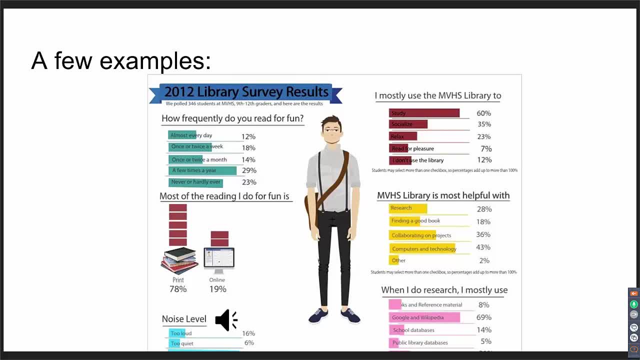 library. so what is just right? that's a good question. that's a good question, Thomas. what is just right? well, apparently, what was happening at that particular library is just right. yeah, it also shows what use the library gets for the most part, as well as what it's. 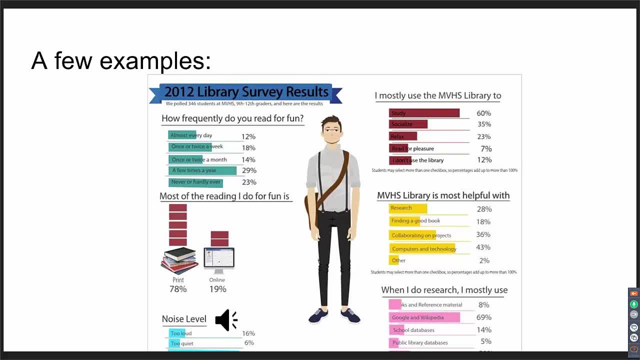 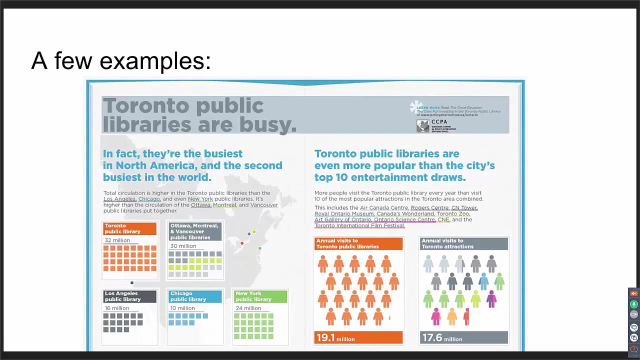 most helpful with, and the tools, the resources that students use when they do research, and so this is just. these are some quick statistics that are interesting. the color helps make it appealing, and it's something that the community your library serves would like to know. here's another example of an 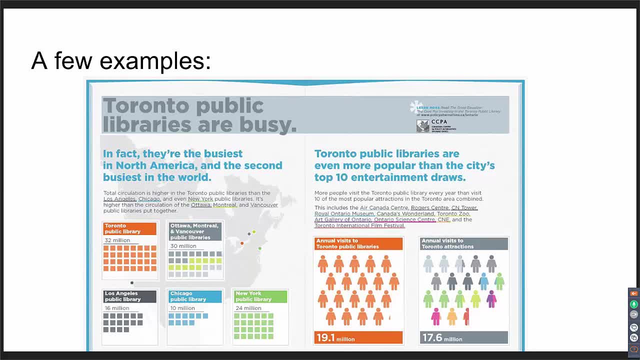 infographic that was made by the Toronto Public Libraries. but what I like about this one is that it's it's simple, it's broken down into two parts. so there's not, you know, there's just two pieces of information. the first is that total circulation. it compares total circulation to other major metropolitan libraries and and 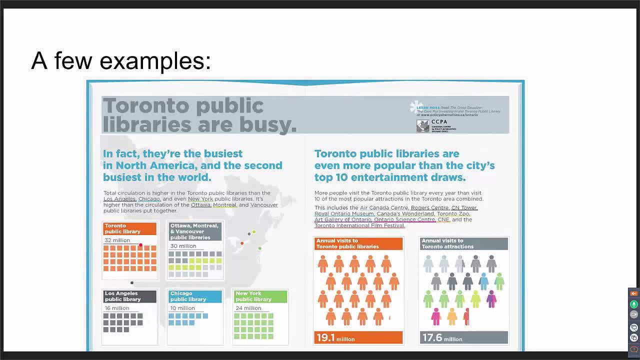 just at a quick glance you can see that the circulation is twice as much as the Los Angeles Public Library, which was very interesting, and it wow, a wow factor there. and in looking at the next part of that, the Toronto Public Library has more annual visits than all of the attractions in Toronto. so just at a quick glance it 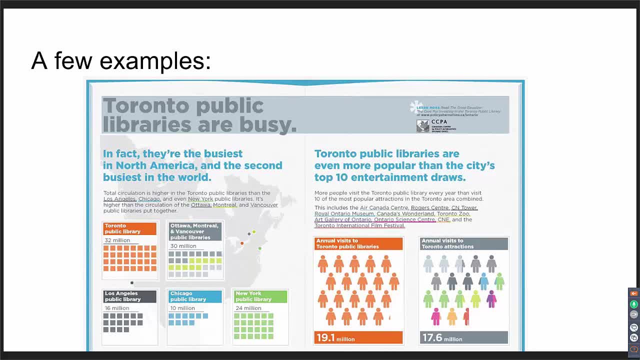 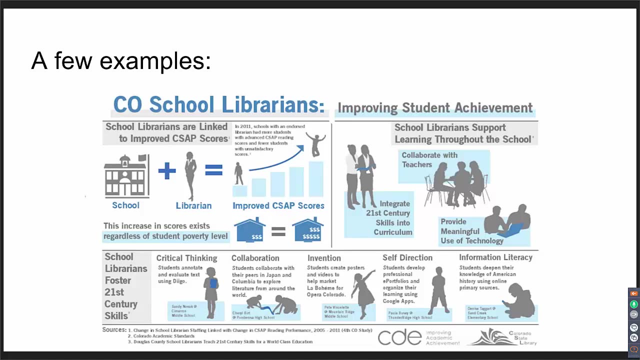 doesn't have to have a ton of information. it can be just a quick sort of a factoid. this might be a little bit more than a factoid, but but those are definitely wow factor. yeah, definitely a wow. this infographic was created by the Colorado State Library and is about Colorado school librarians and their 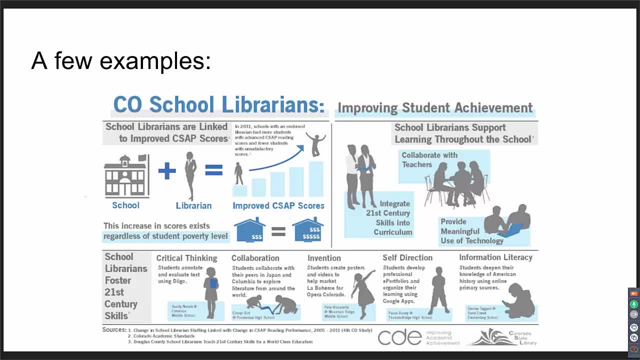 own role in improving student achievement. the important part of this example is that they use several sources of data in order to create the infographic and to tell their story, and they cited the different sources of data that they used. but it isn't just their, their survey. it was pulled from different 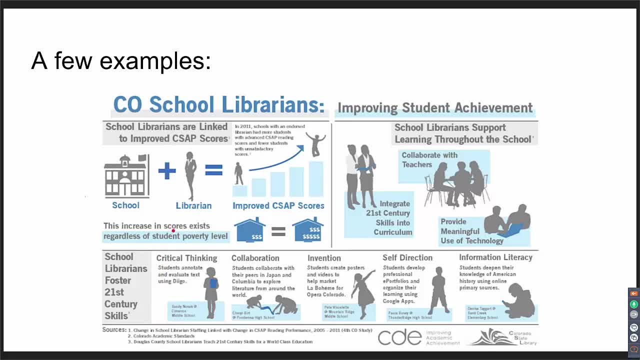 resources, and it just highlights various things that school librarians do to and school library programs do to help student achievement. it's also interesting to note that there are- there aren't any numbers in this infographic. it is text, and so that's another way to to highlight the value that your 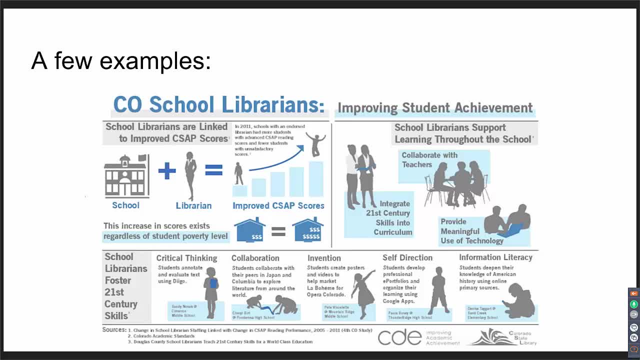 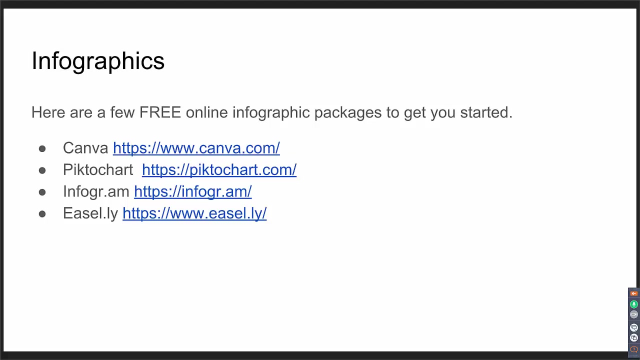 organization brings to your community. it doesn't always have to be numbers, but you can just put in a textual fact and people can read that and it still makes it visually appealing and easy to to digest. so there's a few things to remember. oops, I jumped ahead there. we wanted to let you know that there's a. there are. 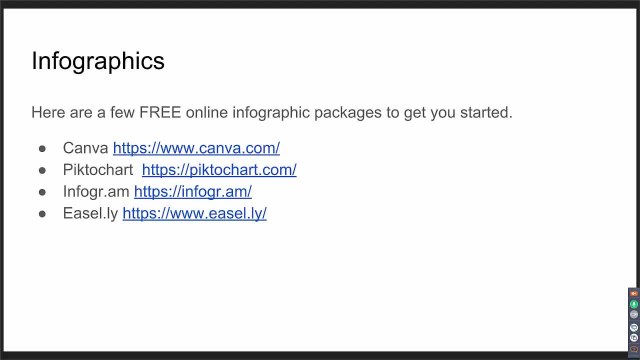 some online free infographic software packages to get you started. it's. it's not all about having aики features, because it's gonna help your package to get you started. it's. it's not aкая methods. so let you start your software package. you get to create the program and select the things that you'd like to do and put in the infographic news. who will help you deliver those? 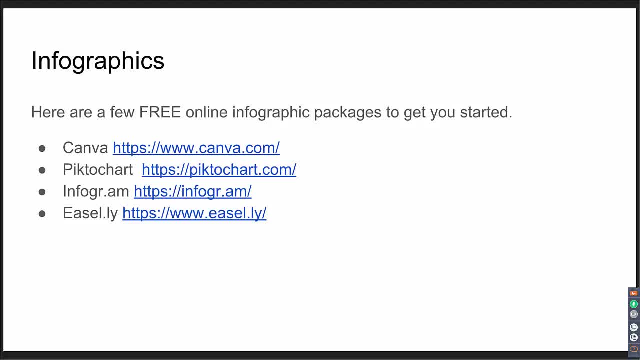 that difficult to create an infographic once you have your source of data and the story that you want to tell. for graphics, for these various ones, some of them have well that, most of them have free graphics that you can use within the program, and templates- yeah, templates- that you can use to make it easy and you 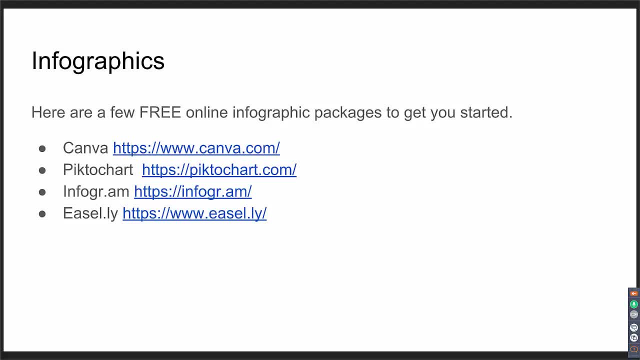 can change colors, so you can get themes, all that stuff. and then they also- some of them- have premium graphics that you have to pay for, of course. so it's like one dollar or two dollars for per graphic, but you, most of them, will let you import your own graphics. so if you have your own that you want to use, let's. 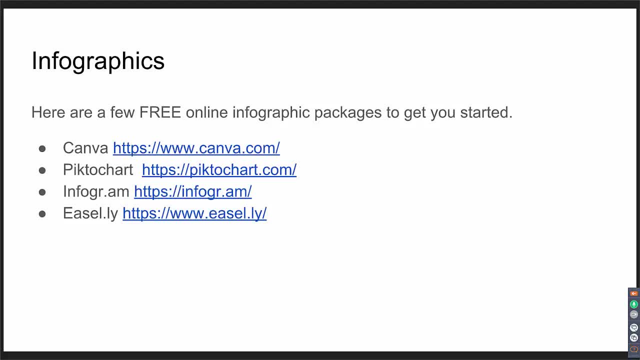 say, if you're doing an infographic on the programs that you've done in your library and you've got pictures of those, you can insert those pictures or you can pull down line art or other copyright free sources from the internet. you can save and use. yeah, you can really. 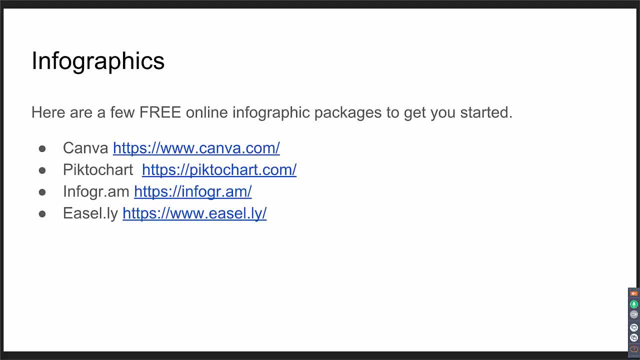 personalize your infographics with these programs and capabilities. oh yeah, and these are just four that we thought we'd share with you. you can come back, revisit the recording if, if you didn't have time to write any of these down, maybe maybe you've used these and you know more of them, I don't know. then maybe you could. 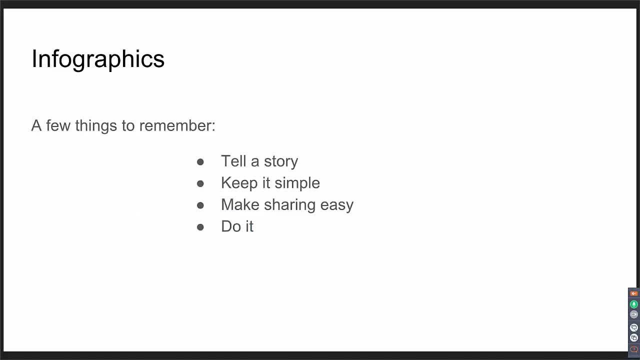 share those with us. that would be great. so a few things to remember about infographics and using your data is that you are, you're trying to tell your story, a particular story I'm. you want to keep it simple and you want to make sharing of it easy. you don't want to make it difficult to share. 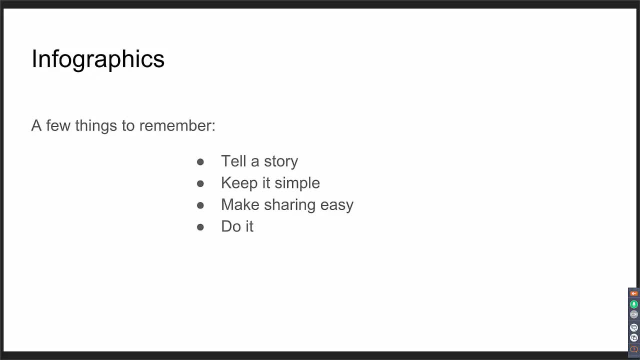 across platforms and the main thing- sometimes the hardest thing, especially when you're new to this, is just do it. you know, and before you publish an infographic, you can play around with it and change it and delete it and start over. but it really is. it's a creative outlet for your data, so don't be afraid. 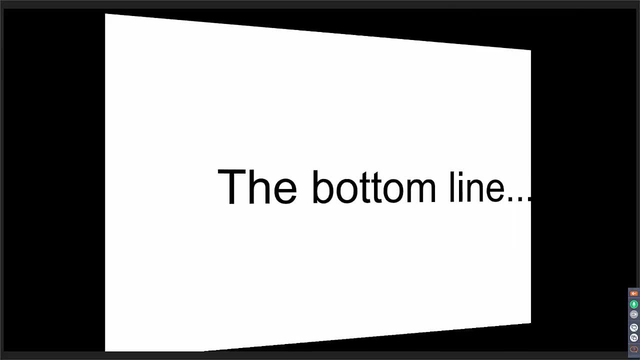 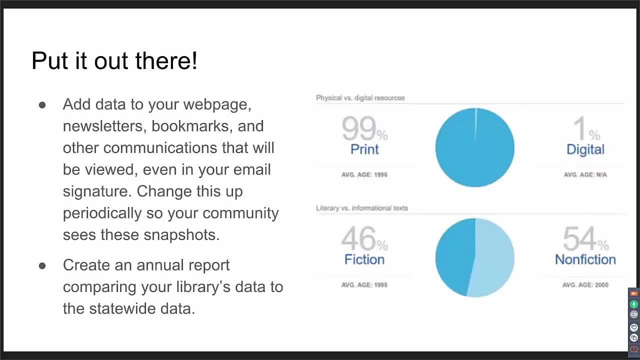 to start with that. so the bottom line: put it out there. you've sorted and analyzed your data and put it into a communicable format, so the next thing you need to do is make sure that people see it. put it anywhere that people will see it and associate it with your library, whether it's public school. 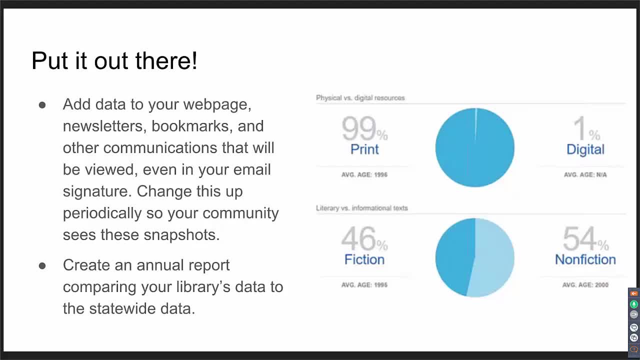 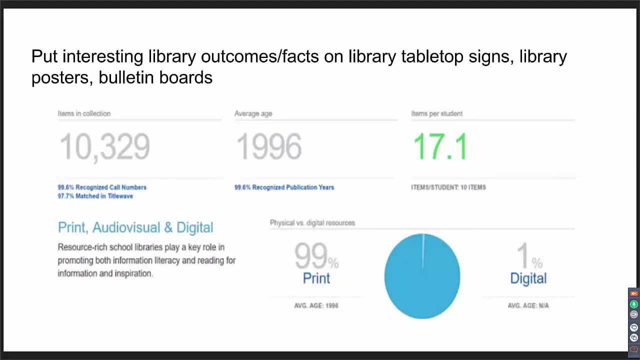 academic or any kind of special library. insert those factoids into your webpage or on circulation notices. your community wants to know. so, plus you took the time to do it, show off the work that you did and get it out there as much as you can. so that's, and you can put interesting library outcomes. 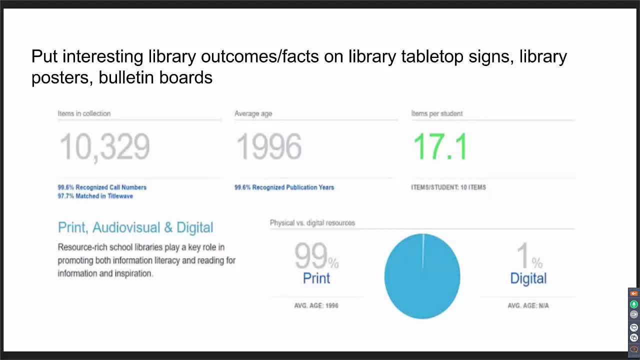 on your public school notepad and you can put out a lot of different articles: tabletop signs, library posters, bulletin boards. you can create an annual report. we've talked mainly about data that's already been collected or that we are collecting at the Wyoming State Library. you can also run quick surveys of your 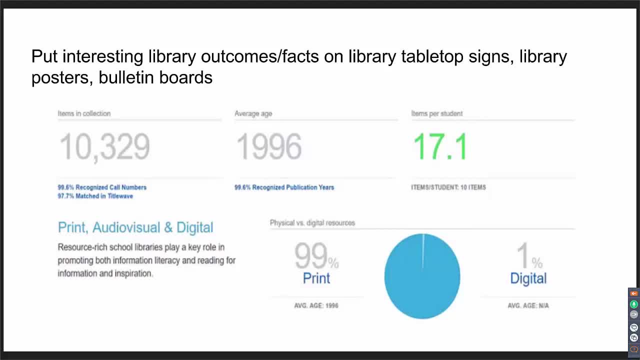 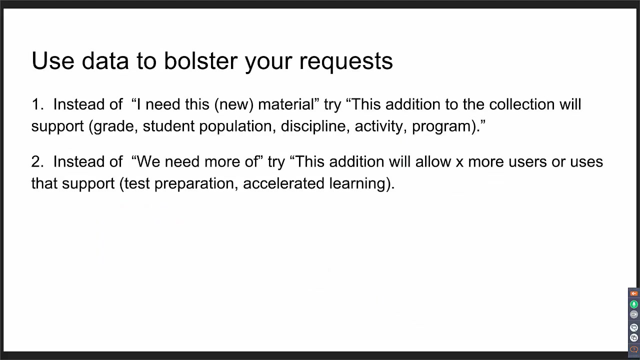 library. you know, maybe asking a question or two and use that data in infographics, but definitely put your story out there. your community wants to know. your community needs to know. they need to know the value of your library to the community and to society in general. show the data to support your requests when. 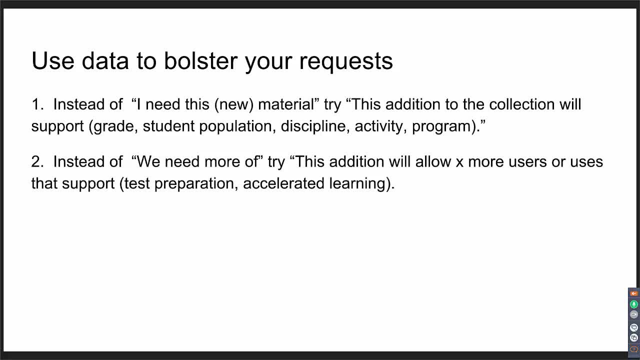 you accompany requests with statistical data, you're also showing the value of your library, so it's important to highlight the positive impact that your library has on the community. so, when doing your requests, instead of saying: you know, I'm not sure about this, I'm not sure about this, I'm not sure about this. 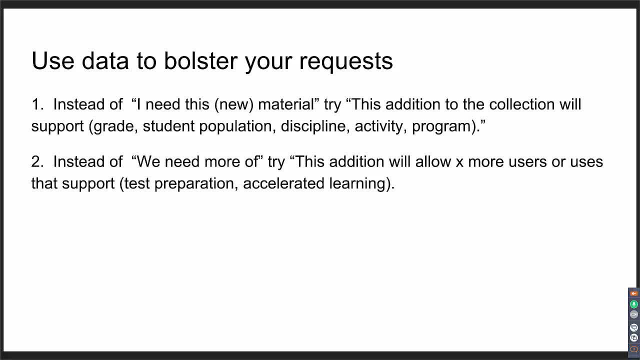 I need this new material. try using something like this addition to the collection supports grade level 11, or the stem program that you're trying to build exactly, or an activity or program, instead of saying we need more of this. try. this addition will allow X more users or uses that support test preparation. 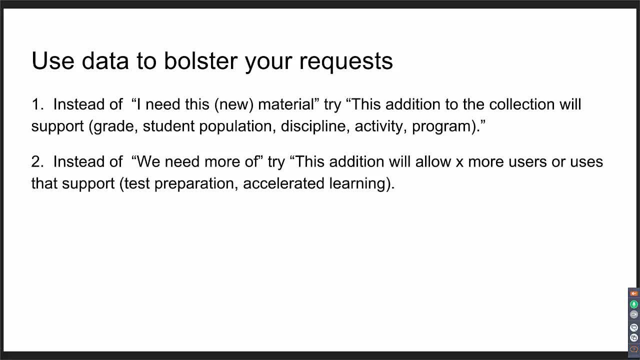 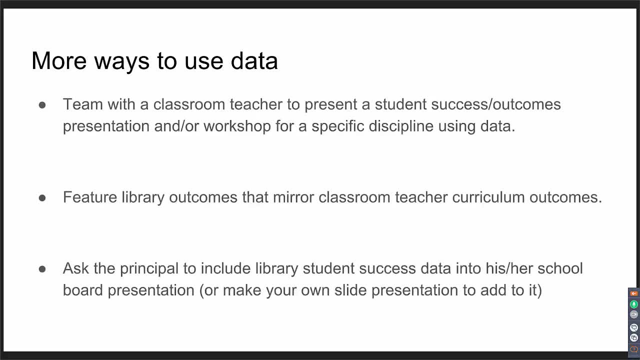 literacy, accelerated learning and show the data that supports your claim. absolutely more ways to use data. our team with a classroom teacher to prevent or to present a student success presentation feature: library outcomes that compare equally with teacher curriculum outcomes. ask your principal to include library student success data in his or her school board. 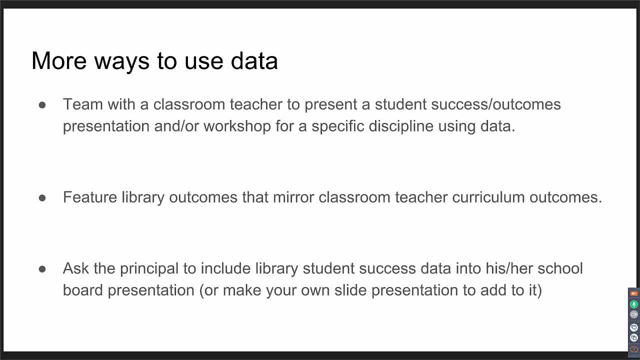 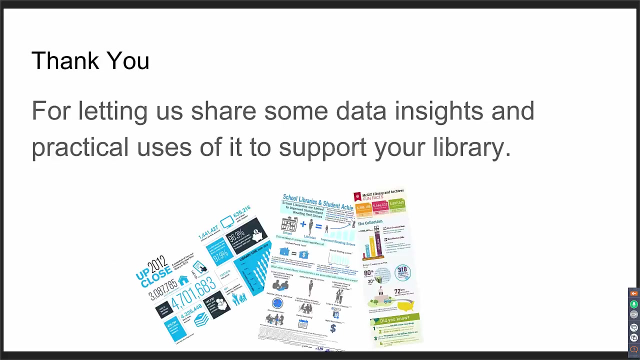 presentation and maybe you can make your own slide presentation that your principal can add to theirs. but the main thing is to remember to be creative. try out different, different ideas and some will work, some may not, but keep trying, never be afraid to get your story out there. so with that, we'd like to thank. 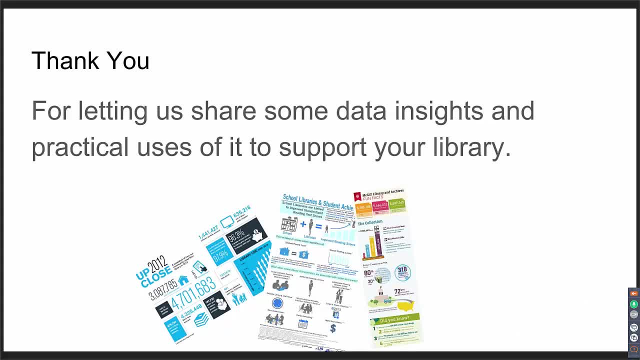 you for letting us share some data, insights and practical uses of it to support your library and your students. our next webinar will be on the Wyoming State Library and we don't want you to forget that this webinar will be available on the Wyoming State Library YouTube channel and you can revisit it anytime, and I believe there will be PDF. 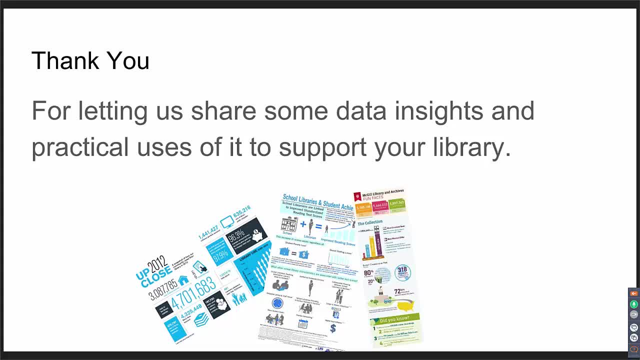 as well. yes, Thomas, there will be a PDF available on the Wyoming State Library website, along with the archived link, and you'll be able to access it with the YouTube video when you go to YouTube. now call the camera and let me know if you've got any questions or anything you'd like to ask. you can always call the camera on the watch and we'll be happy to answer any questions, and any questions you have are. there are no questions from the audience. if there are any questions that you want to ask, we'll be happy to answer them. 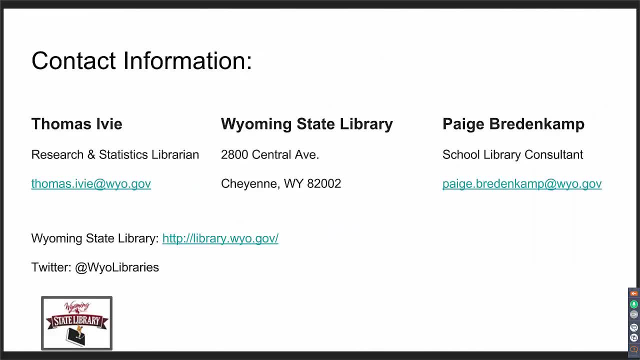 Thanks, contact information here. you can contact Thomas or myself, and you can also get on to the Wyoming State Library website or find us on Twitter. we use Twitter a lot. it's a great way to communicate and thank you for attending. now we will take questions. if anybody has any questions about today's presentation, okay, do you? 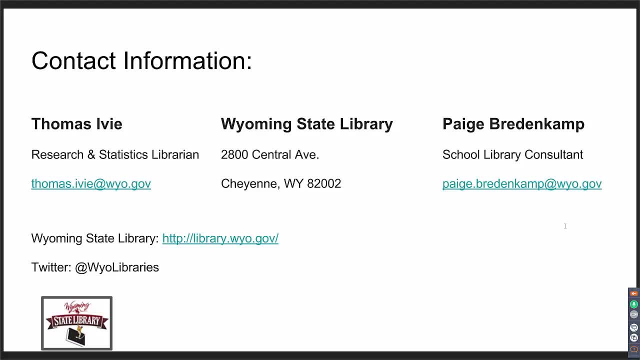 use a specific program to create the infographic I do. I use I like using canva, but my process is I'll have a list of programs and their websites and I start with one. if I don't like it, I move on to the next one, and I think in this: 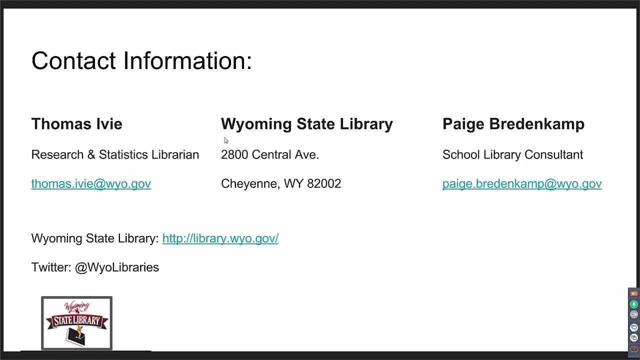 case, I did do that. I started this one I didn't like it moved to the next one, which happened to be canva, and once I find something I like and I just stick with it, but it's kind of it's a preference thing. once you what.